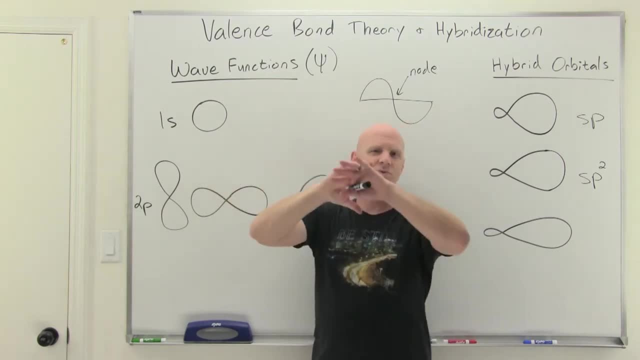 start having these radial nodes areas at a set radius around the nucleus where you also won't find an electron. So that's kind of what we're going to look at here, And then we're going to look at the 2s and the 2p, But I'm gonna leave those out of the discussion. I really just want. 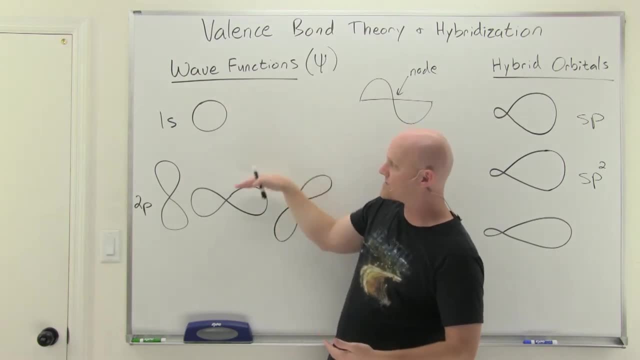 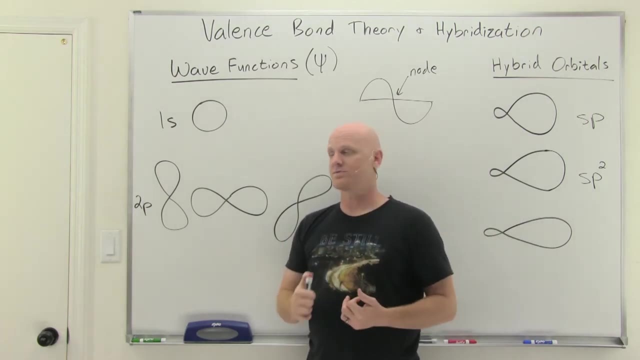 to focus here. But the big thing: take away from those that as you go to higher orders of s and p orbitals- higher shells if you will- they're larger and they end up forming longer bonds, which are typically weaker bonds and things of this sort. All right, one last thing to talk. 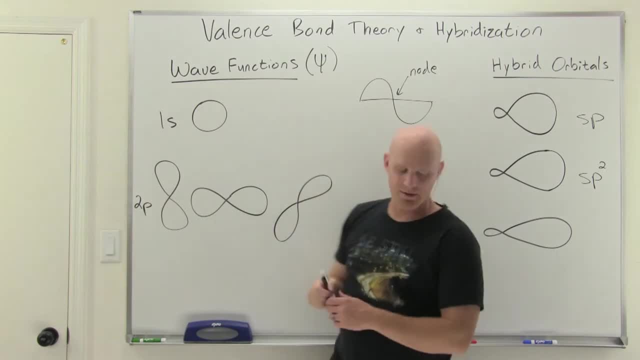 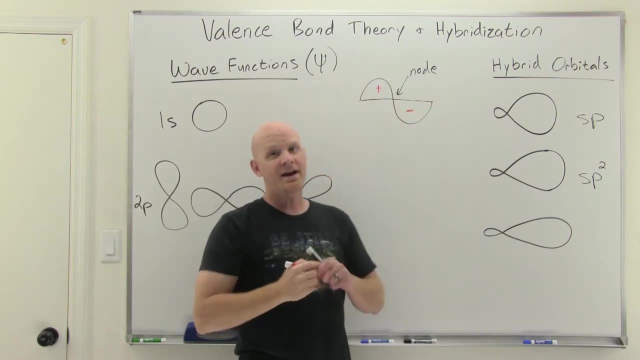 about with these wave functions. So, just like a sine function can be both positive and negative, and notice, from zero to pi your sine function is positive and from pi to two pi, your sine function takes on negative values. And every time you cross from positive, negative, 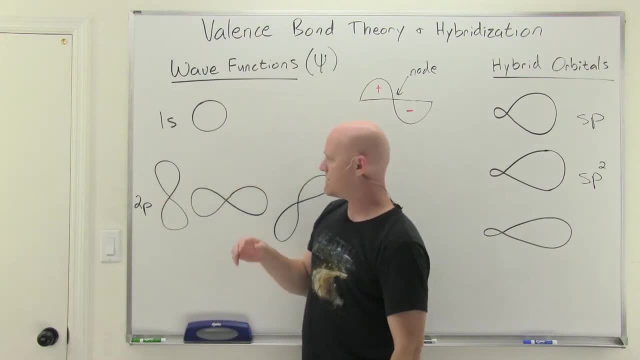 you got to cross through zero and that's your node. And so same thing here. if we look at that p orbital right at the nucleus, whether it be the, the p orbital on the y axis, the x axis or the z axis, that's the difference in those three p orbitals. So they all have a node right at the 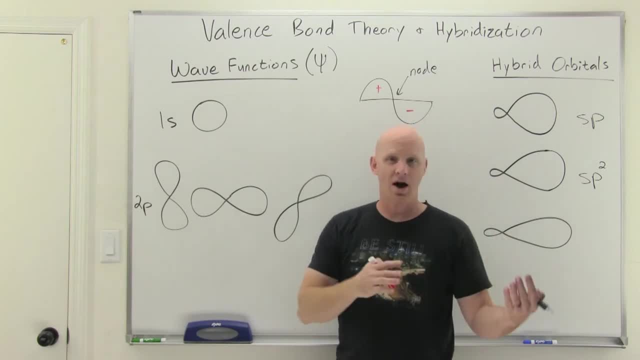 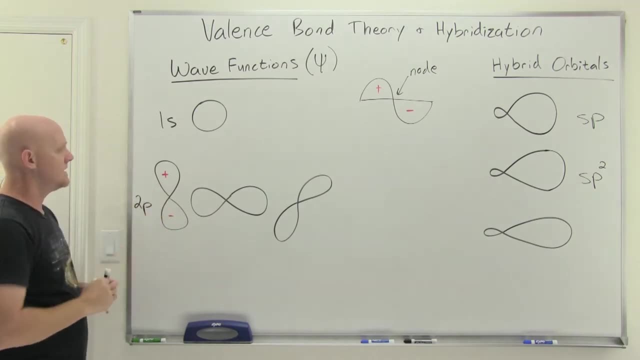 nucleus, And the reason they have that node is that your function is going from positive to negative, And it might be positive on top and negative on bottom, or vice versa. it's totally arbitrary for this lovely p orbital on the y axis, And so sometimes, instead of showing plus and minus, 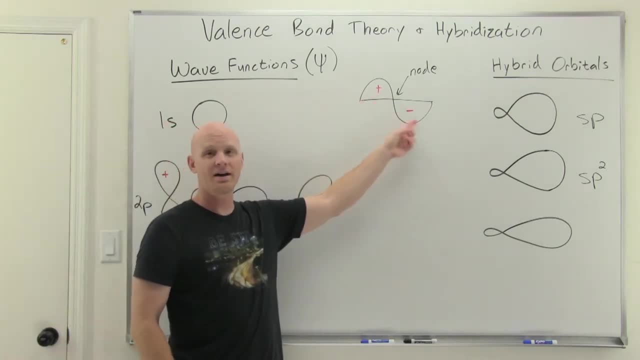 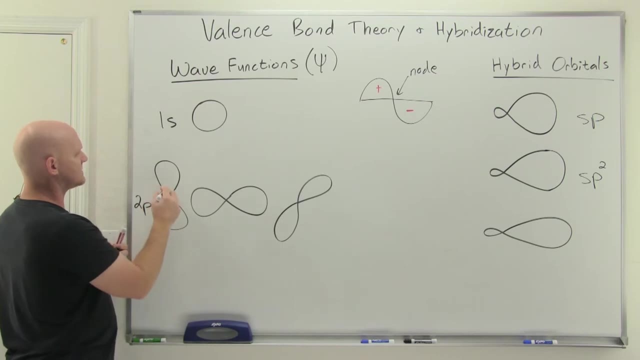 and again, this is not charge, this is the particle sine, just the values of the function itself. So in this case, and sometimes, instead of actually showing the plus and minus, sometimes what we do is actually do a difference in shading. we'll shade one side and not shade the other, or shade one side- blue, and shade the other side, green. 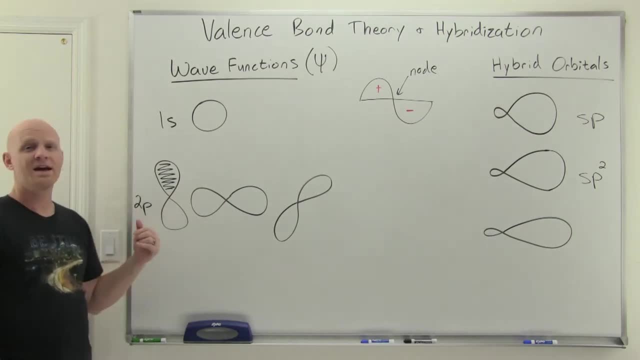 or something along these lines. So here I'm just using one side shading and one side not shading, And it's not like one means plus and the other means minus, But one of them does mean plus and the other minus. it's just arbitrary which is which. So this just shows you that there's two. 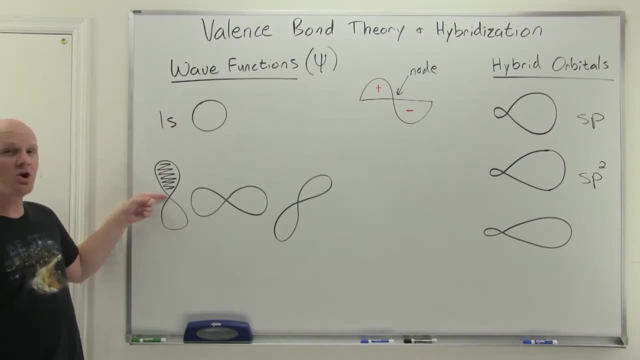 different signs for the different sides of this wave function. And then again that node right at the end of the nucleus Cool, So again at the heart of valence. bond theory is overlapping orbitals to create these covalent bonds. Now, if we take a look at a very simple molecule to start off, 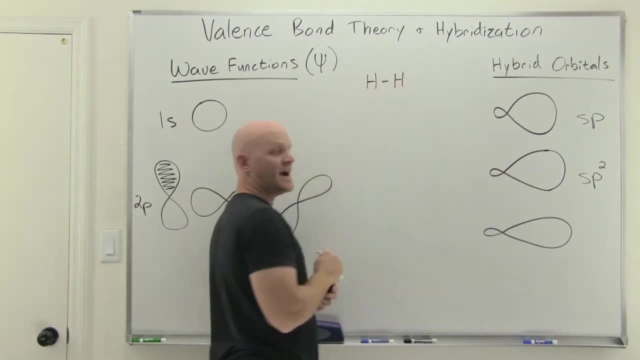 with, and we'll just start off with, a molecule of elemental hydrogen, here, H2.. So that lovely line represents a covalent bond, And what we actually really have going on is so hydrogen's got its unpaired electron, its only electron, in an s orbital, And those s orbitals are going to come. 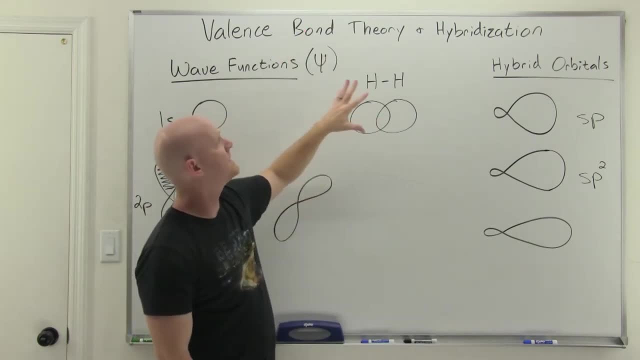 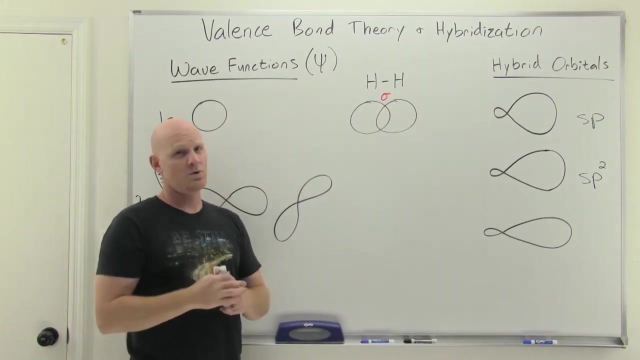 together and overlap according to valence bond theory. So that's where, in these overlapping orbitals, that's where the electrons are going to live, that are being shared here, The ones described by that lovely line there representing the covalent bond. So, and it turns out we would call this a sigma overlap. So we'll get exactly what that means here. 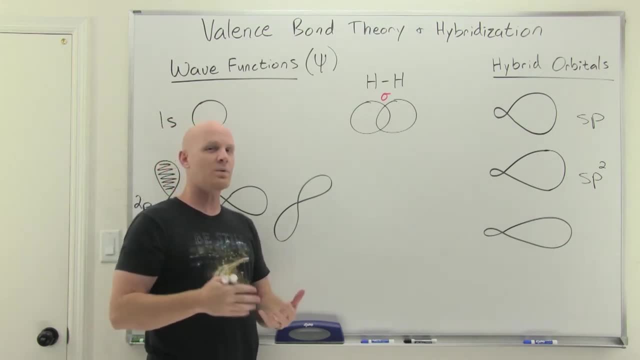 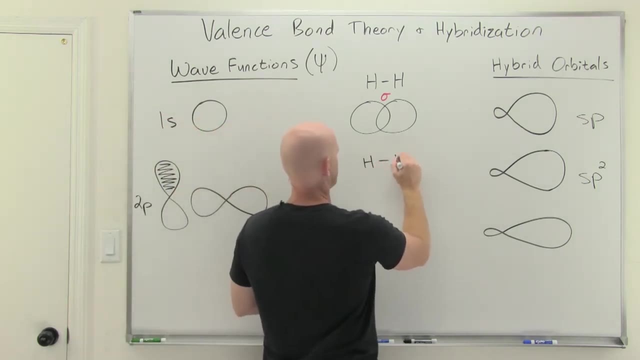 in a second. So often it's not going to be easy to identify what it means until you see something that's not an example. We'll see pi overlap here in a little bit. If we compare this to say HF, So hydrogen again. 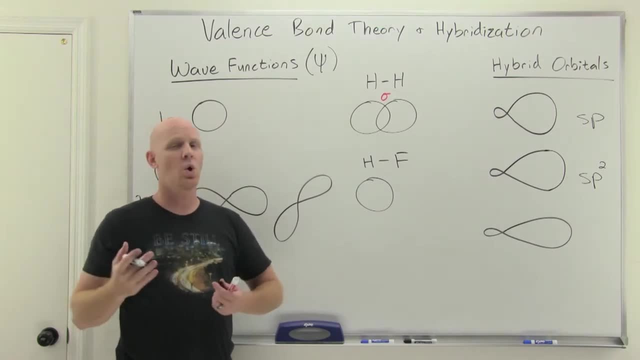 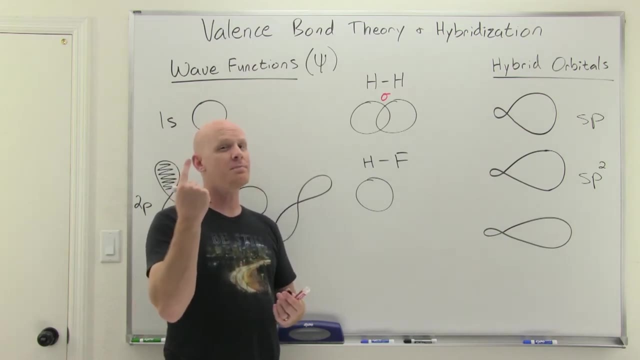 has an s orbital here, so that it's one s electron. it's only electrons involved in So. but fluorine, his valence electrons are in the 2s and the 2p, So and in this case his unpaired electron. so valence bond theory talks about atoms using their unpaired electrons. 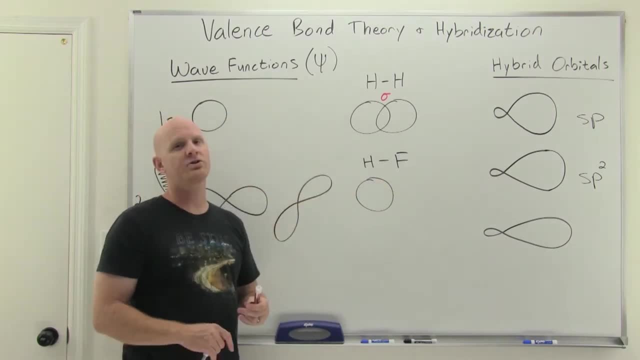 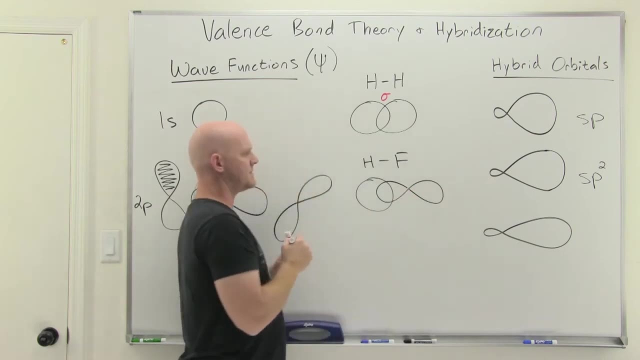 those are the ones they share. Well, for fluorine, its unpaired electron is in one of these 2p orbitals, And so fluorine here is going to overlap its 2p orbital with hydrogen's 1s orbital. I've probably drawn the 1s a little big, or the 2p. 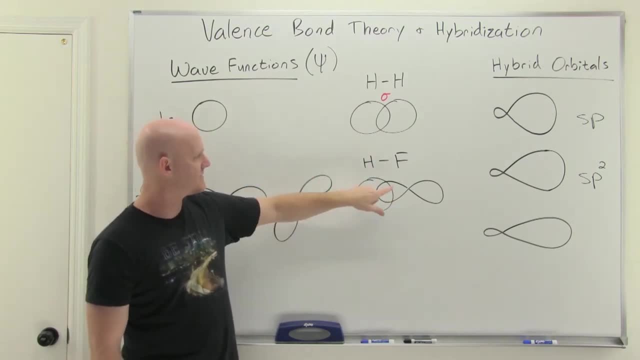 a little smaller, But it's going to overlap its 2p orbital with hydrogen's 1s orbital. I've probably drawn the 1s a little big or the 2p a little smaller- small truth be told, but you get the idea. And again, in these overlapping orbitals, 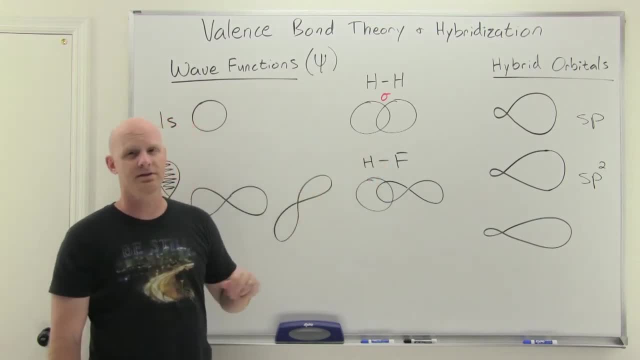 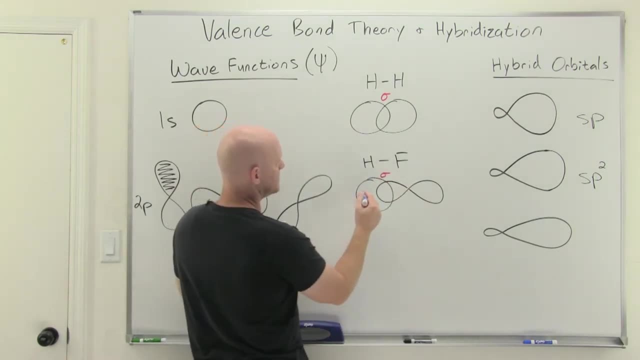 that's where our lovely two shared electrons are going to live. That again is valence bond theory And again this is also described as sigma overlap. Now if I take a and highlight in blue where the nuclei are in both cases here, what you find is that we say that the overlap 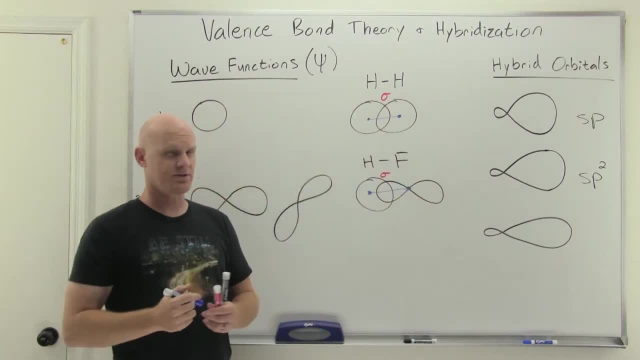 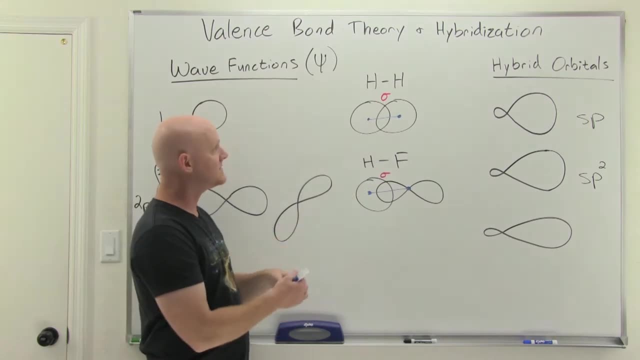 occurs along this inter nuclear axis- that's our technical term And it's just the line connecting the two nuclei. And as long as your orbital overlap is occurring somewhere on that line, that is sigma overlap And it turns out they give it the letter sigma. 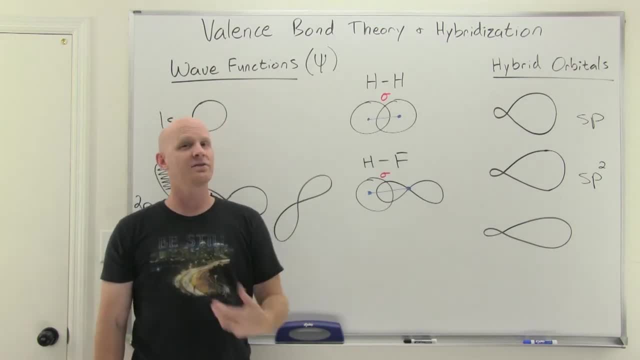 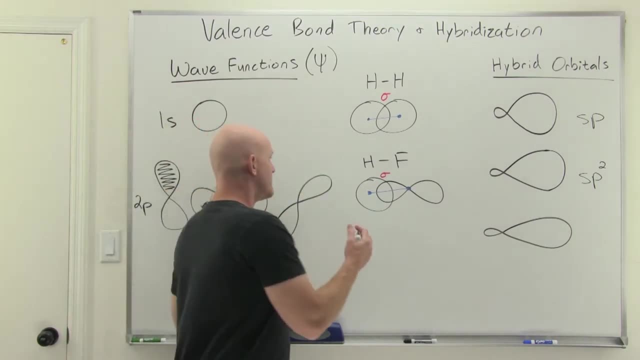 here, That's the Greek letter sigma, which corresponds to our English letter s, And it's because all single bonds are sigma bonds, as we'll find out in a little bit Cool. Let's look at one more example of this, And maybe if we look at a molecule of F2.. So in this case, both of them have. 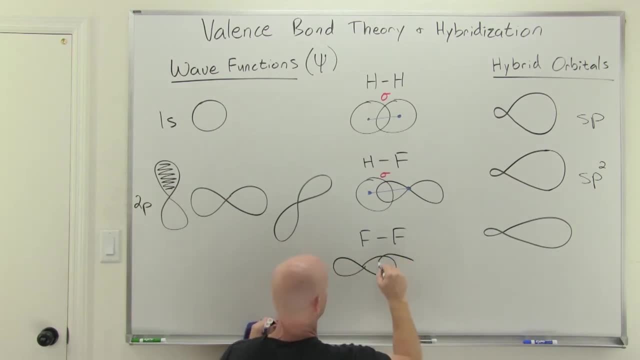 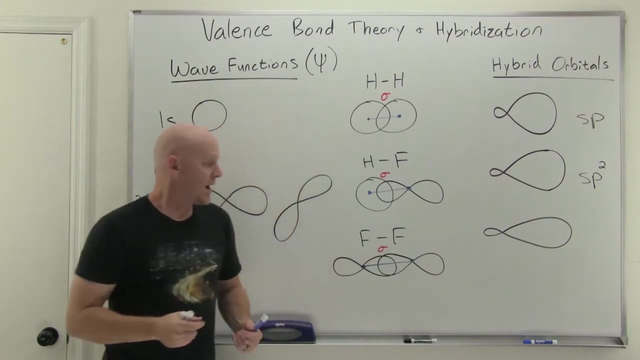 their unpaired electrons in s orbitals, And so your s orbitals are overlap sideways here, And once again that overlap is occurring along this inter nuclear axis, And so once again, we will refer to this as being sigma overlap. Cool, Now, pi overlap is the only other type that 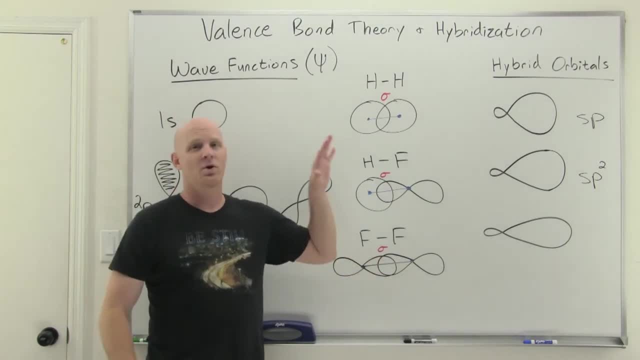 we'll talk about in this course. there's sigma and there's pi, and that's it, And so pi is nice. So for a sigma overlap you can use any kind of orbital. So you can use s's, you can use an s, and 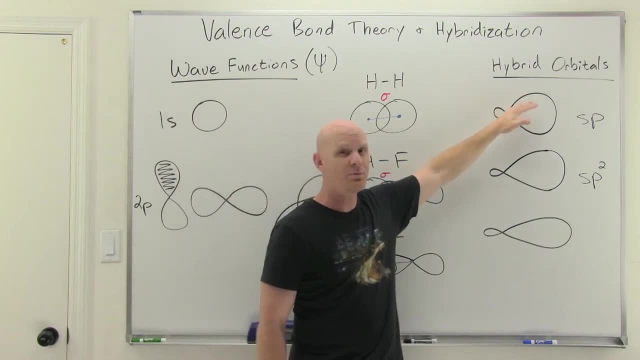 a p. you can use a p and a p. you can also use these hybrid orbitals that I'll reference a little bit later, But we have sp, sp and sp. So you can use s and a p. you can use a p and a p. you can also use these hybrid orbitals that I'll reference a little bit later, but we have sp, sp and sp. 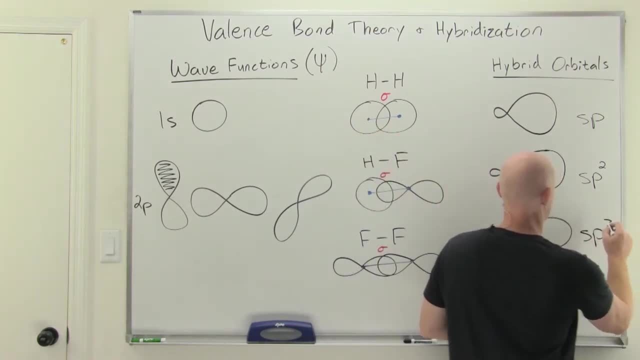 So you can use s and a p. you can also use these hybrid orbitals that I'll reference a little bit later, but we have sp, sp and sp- And I didn't write it down here- sp- three hybrid orbitals. Those can also be used in sigma overlap as well, But pi overlap is specific. 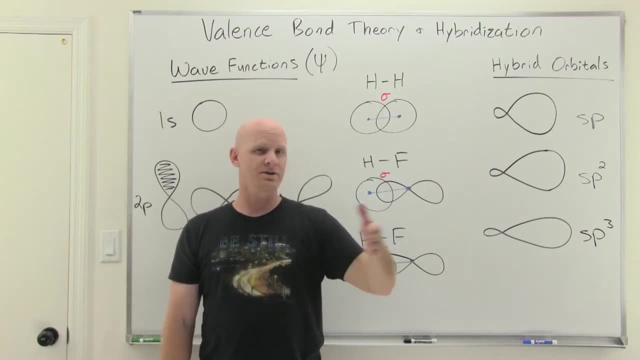 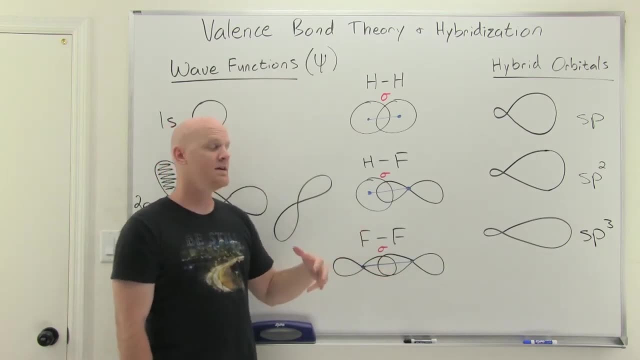 And pi Greek letter p essentially so it corresponds to our English letter p and you could only use p orbitals for pi overlap. But we used p orbitals here and that was still sigma overlap. So the key is: it's not end to end overlap, It's not overlap that's going to take. 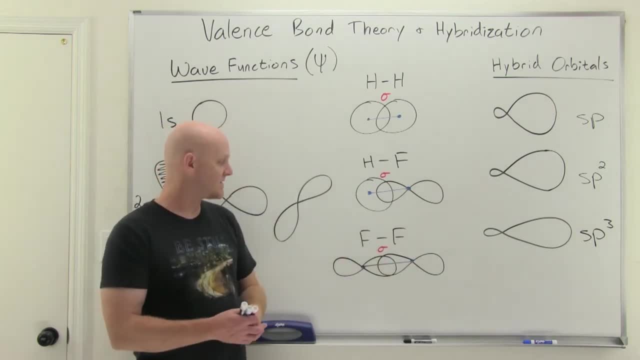 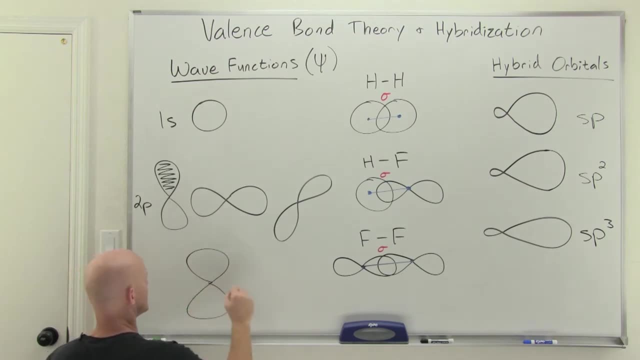 place on this inter nuclear axis. It turns out it's going to be pi. overlap is going to be when to side. Let's do it where we've got a little more room here. So we've got two atoms next to each other. So again, here's our nuclei, But the overlap doesn't occur along this internuclear. 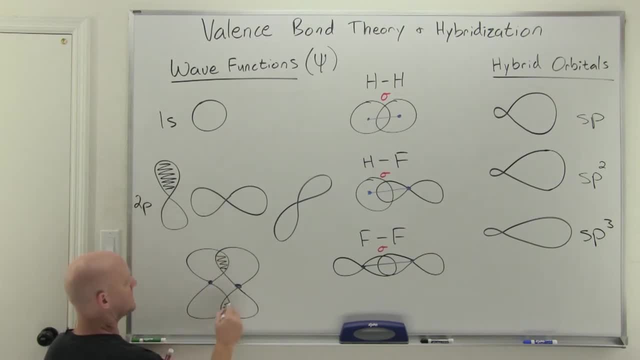 line, The overlap's occurring above and below that internuclear axis, And so that is what we refer to as pi overlap Cool, And the only orbitals allowed to be involved are p orbitals, and they overlap side to side, not end to end. we say So in summary: the end to end overlap of. 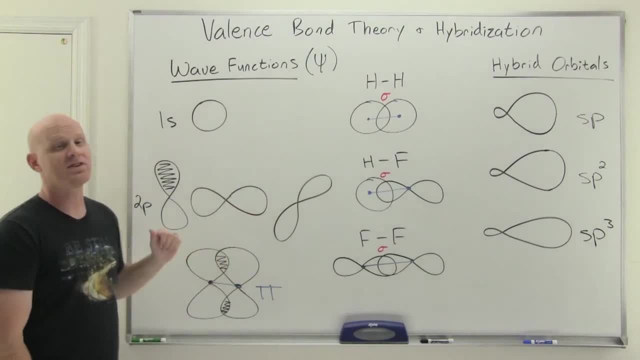 any two orbitals. that's going to be sigma overlap, But the side to side overlap of p orbitals and only p orbitals. that is our pi overlap, And we'll find out. we're only going to have pi bonds with double and triple bonds. So it turns out when you start making multiple bonds it turns out you're. 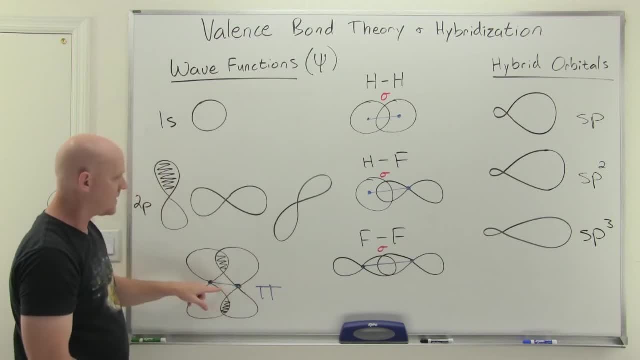 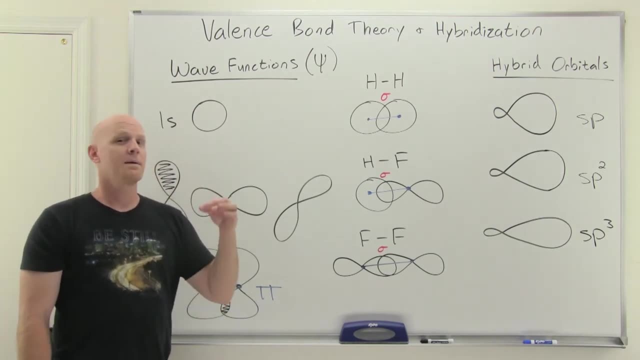 only going to have one set of orbitals that actually point towards each other along this internuclear axis. So just like here, here, here, And so you can only make one sigma bond, and that's the first one any two atoms always makes. But if you're going to make any additional bonds, then it can't. 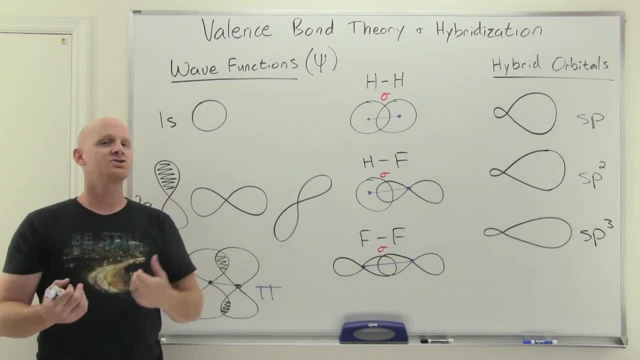 be along this internuclear axis where you're already making a sigma bond. Any additional ones are going to have to be sideways overlap of p orbitals. So a double bond would be one sigma and one pi. a triple bond would be one sigma and two pi bonds. All right, so now I'm going to take 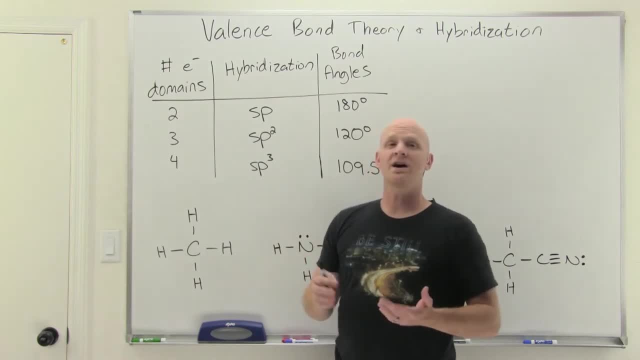 a little bit deeper look at hybridization. And so first off, I just want to point out that you can just look at a Lewis structure and determine an atom's hybridization without even understanding what hybridization is. So I want to point that out first, because you definitely 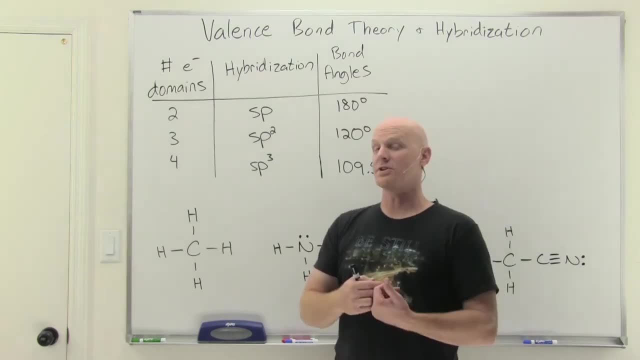 have to know what hybridization is, And so I'm going to point that out first, because you have to be able to quickly determine hybridization, And the truth is, you don't really need to even understand hybridization. to pull that off Now, you will have to have a little bit better. 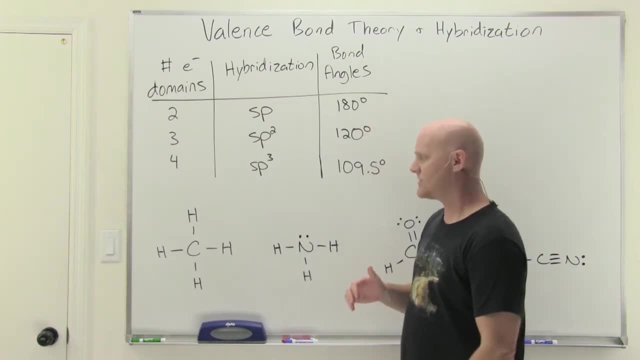 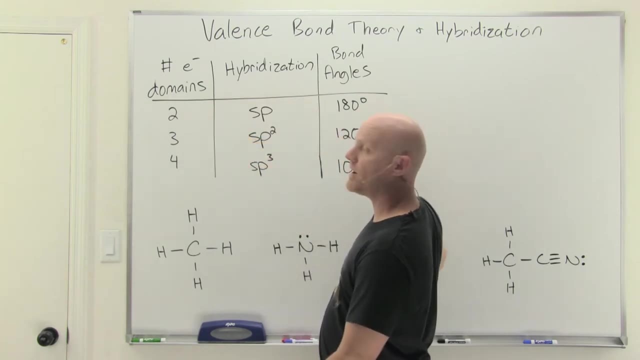 understanding of hybridization, and we will get into that in a little bit So, but it turns out there's a simple relationship between the number of electron domains around an atom and its corresponding hybridization, as well as its bond angles, And we related this back to like VSEPR. 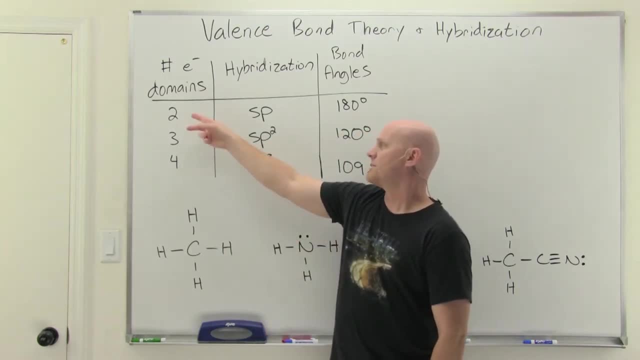 theory in Gen Chem and things of that sort, And we said that. so the farthest apart you could put two things is 180 degrees. And so valence, shell, electron peripulsion, VSEPR theory says the electron domains around an atom want to spread out as far as they can, And so you can put two things and 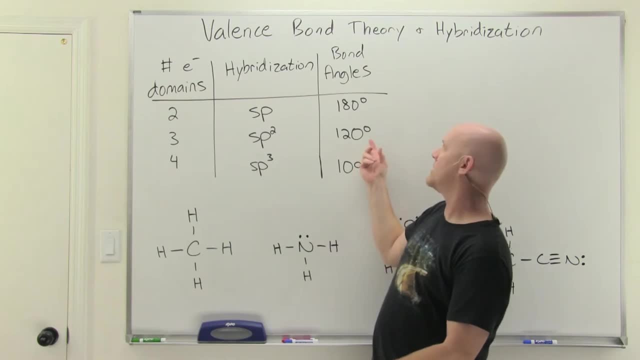 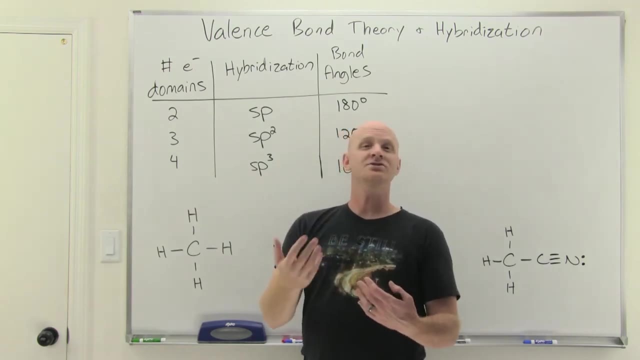 that's 180 degrees. For three things, it was going to be 120 degrees, So that corresponds to a trigonal planar shape, whereas the 180 was linear. And then, finally, for four things, it spreads out into a three-dimensional shape, Instead of being 90 degrees apart, in three dimensions they can. 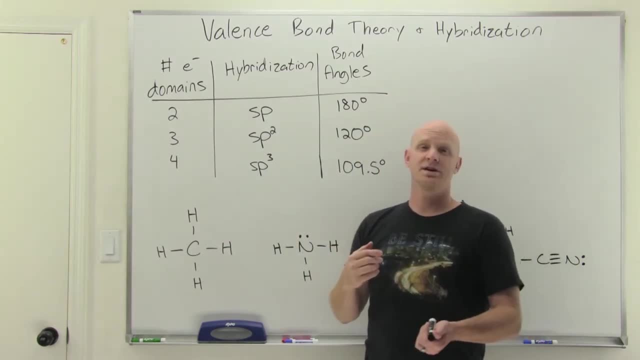 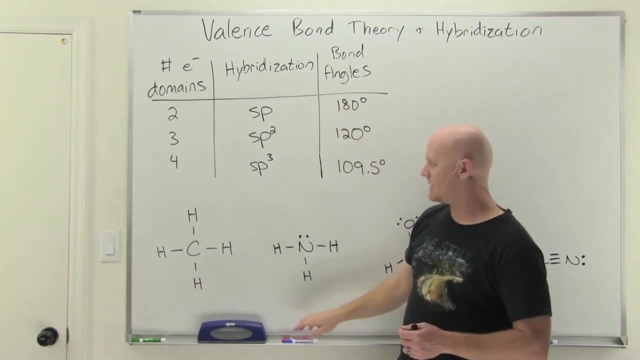 spread out a little further to 109.5 degrees apart in a tetrahedral shape, And you can also relate this to corresponding hybridizations. Now again, we'll get into what those mean a little bit later and give you a little bit better understanding. But if we look at this, we first got to talk. 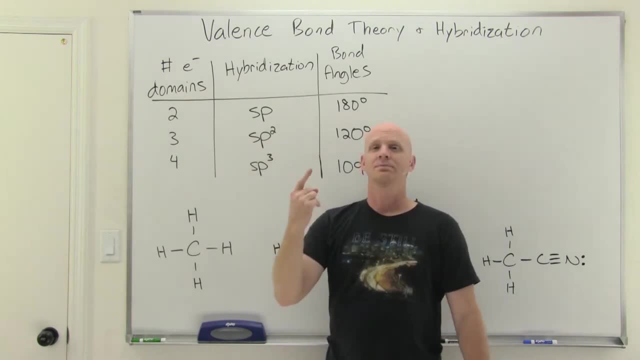 about what is an electron, And we're going to talk about what is an electron And we're going to talk about what is an electron domain. An electron domain is one of two things. It's either an atom that you're bonded to- and I say you an atom that another atom is bonded to, or it's a non-bonding. 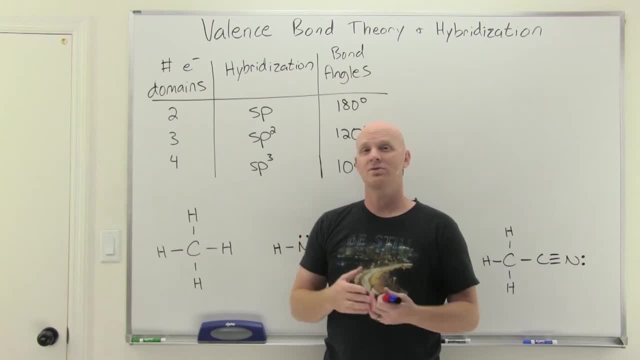 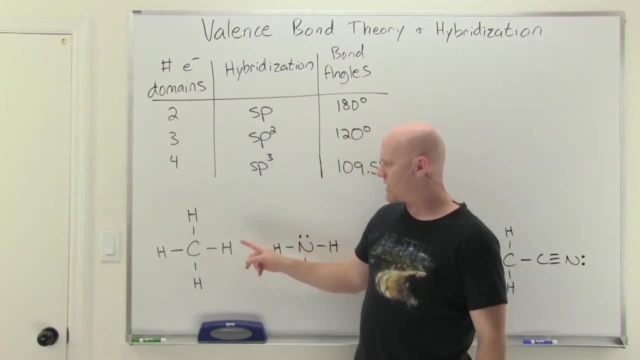 pair of electrons. That's it. And when we say an atom, that an atom is bonded to, it doesn't matter if it's a single bond, a double bond or a triple bond. that is still just an electron domain. So, for example, this carbon right here is bonded to four different atoms directly and has no lone. 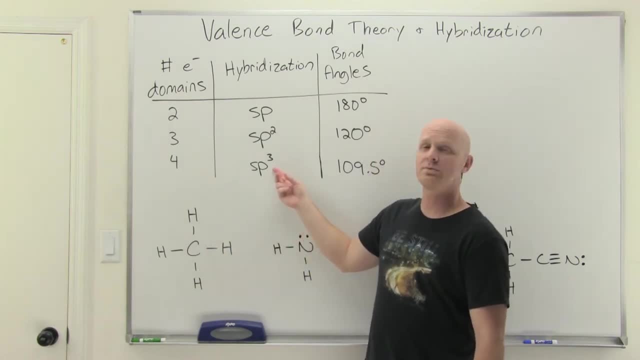 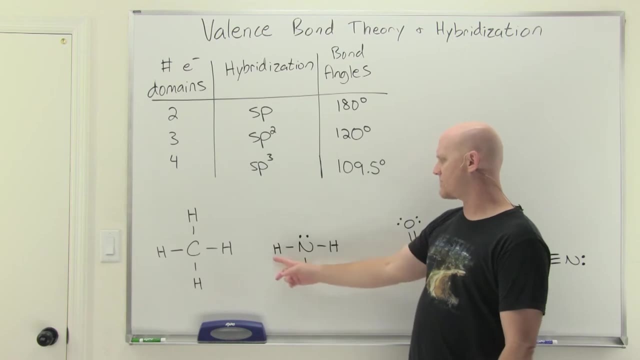 pairs, That's a total of four electron domains. Its hybridization will be described as sp3 and its bond angles would be 109.5.. Okay, so we'll move on to the next one. So we're going to talk about right here. So nitrogen: here's got three atoms it's bonded to and one lone pair, also for a total. of four electron domains. So the nitrogen, we'd say, is sp3 hybridized, and its bond angles are roughly 109.5.. Now, the truth is, though, so with this 109.5, it turns out that the lone pair gives greater repulsion to the electrons in this bonds than they do to each other, And so they get scrunched down. 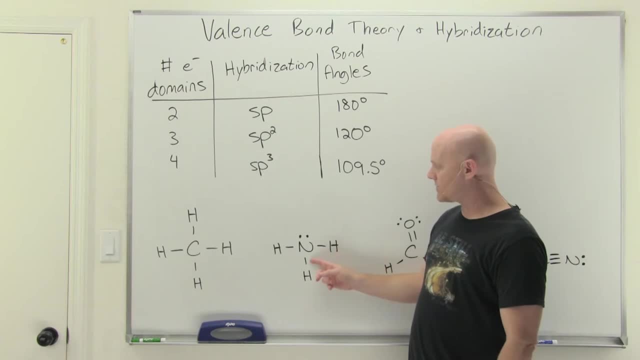 a little bit, and you should know that that occurs. And so the bond angles here, the angles between the actual bonds, instead of being 109.5 exactly, is just a teeny bit less. Turns out right around ammonia, and you wouldn't be responsible for knowing that it's 107, but you should know that. 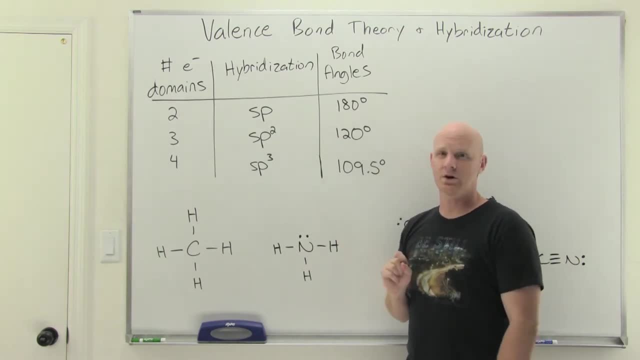 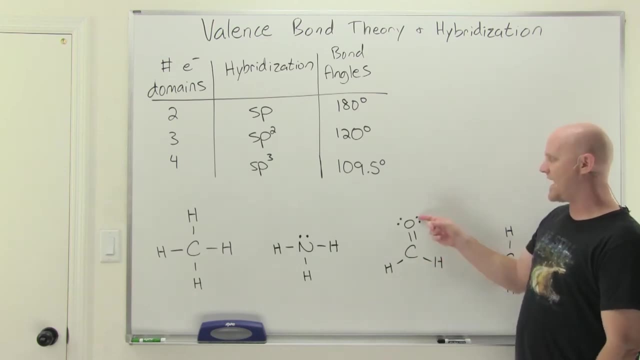 instead of being exactly 109.5, it is just slightly lower than 109.5.. Cool. Look at the next example here. This is formaldehyde, And in this case the carbon is bonded to three atoms. It doesn't matter if this is a double bond, We're just going to count that as one electron domain. 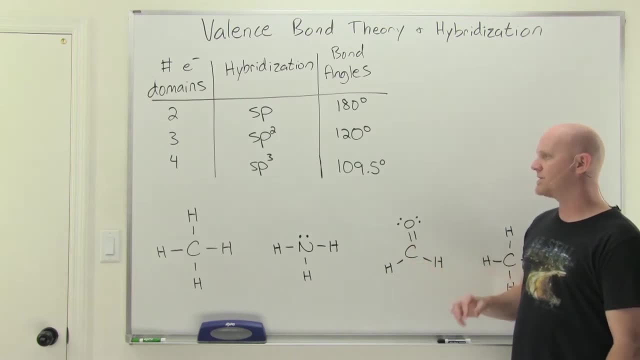 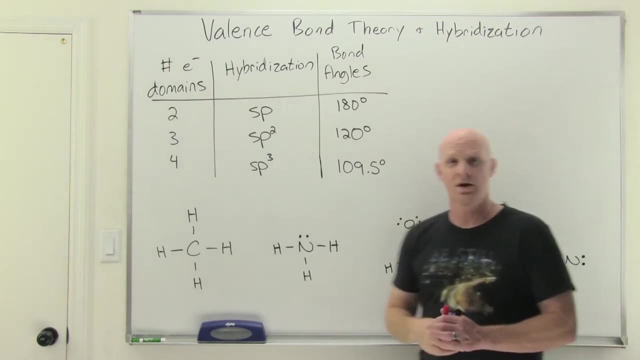 So one, two, three electron domains total because there's no lone pairs around the carbon. And with three electron domains we'd say that that carbon is sp2 hybridized and that the bond angles around it are going to be 120 degrees. Now here's another place where the bond angles won't be. 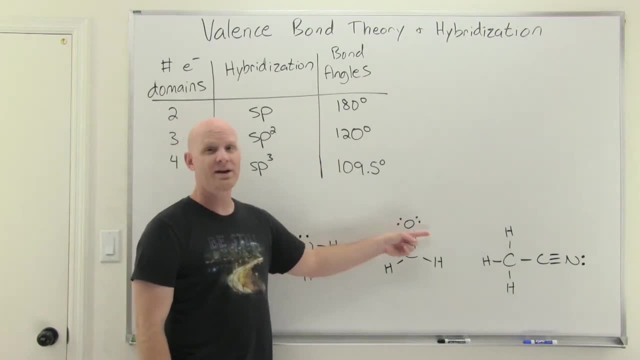 exactly the number listed here, because this double bond has greater electron density than the single bonds, And so there's going to be a greater repulsion, And so the angle between the double and the single actually slightly bigger than 120 on both sides, And that forces this. 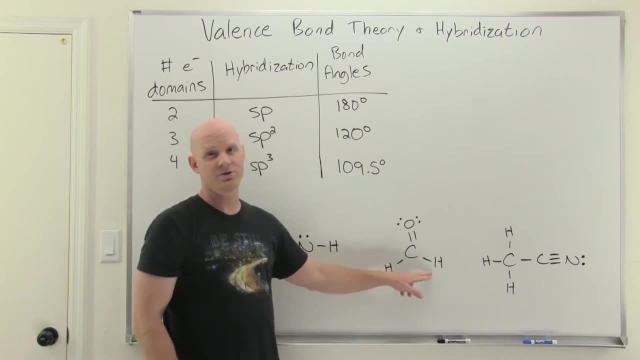 which gets scrunched down just a little bit to be a little bit smaller than 120 degrees. Now we could say again that the bond angles are approximately 120, and that's a true statement. but they're not exactly in this case as well, because one of the electron domains was a double. 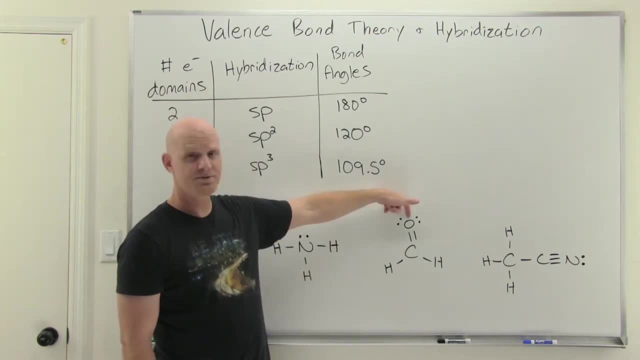 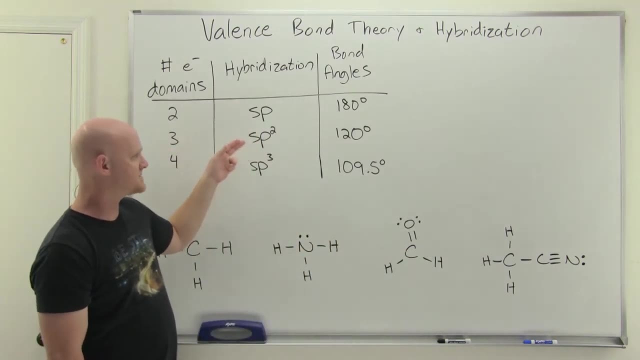 bond, whereas the others were singles. Cool From Auction's perspective. Auction is bonded to one atom and has two lone pairs, Also for a total of three electron domains. the Auction's sp2 hybridized and the bond angles, if it had multiple. 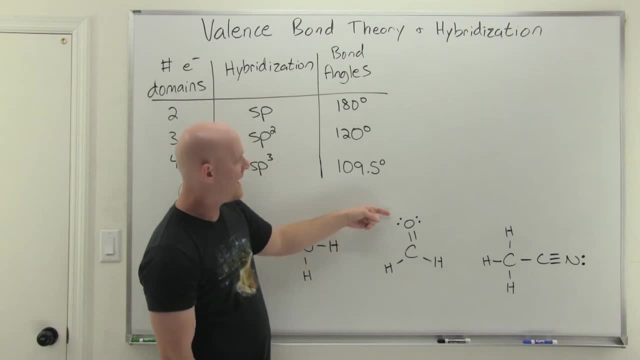 bonds in this case would be 120.. Well, in this case it doesn't actually have multiple bonds, but the angle you could say between the lone pairs is 120, or between the lone pair and the lone would be 120, but that technically wouldn't be a bond angle, but it would be roughly 120. 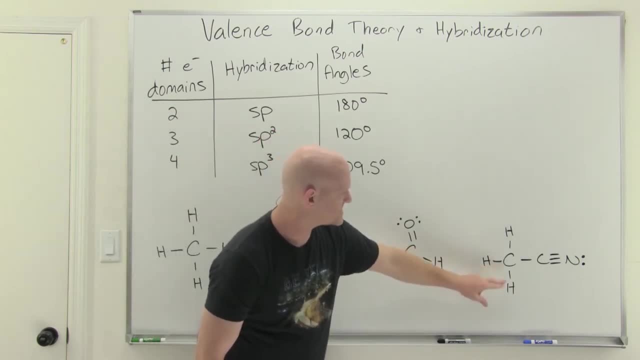 Finally, on this last one, we could look at a few different atoms. We could look at the carbon on the left which is bonded to four different atoms and is sp3 hybridized- 109.5,. we could look at this carbon right here which is bonded to two atoms and is sp hybridized and bond. 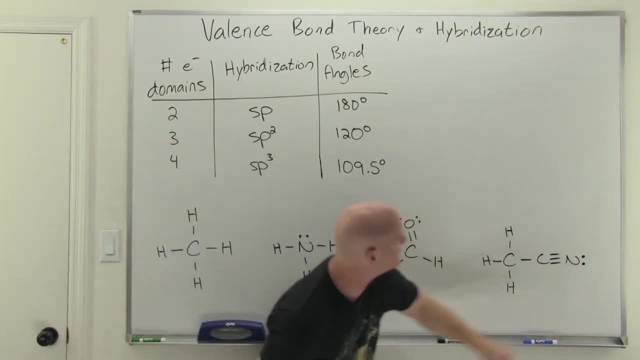 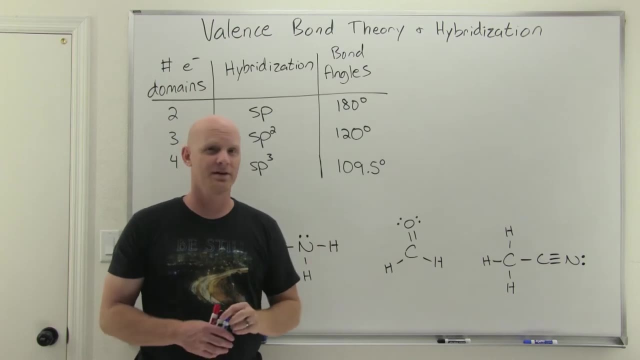 angles of 180.. And then we can look at the nitrogen, which is bonded to one atom and has one lone pair, also sp, hybridized. Cool, That's how you can identify an atom's hybridization: simply by looking at it and counting the number of electron domains. We'll see where this comes from in a. 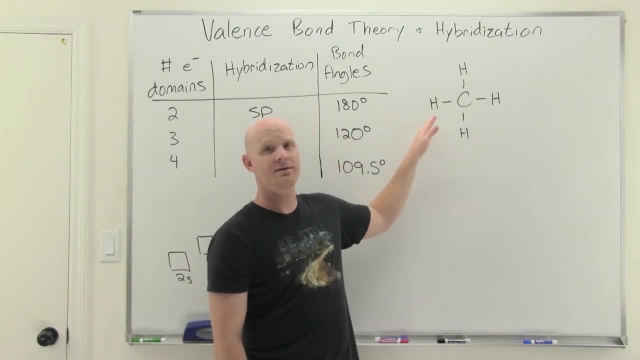 little bit Okay. so I want to take a little closer look at methane here to kind of get the idea of where this- you know idea of hybridization even comes from. So in this case we see that carbons bonded to four different hydrogens. So and for bonding theories, 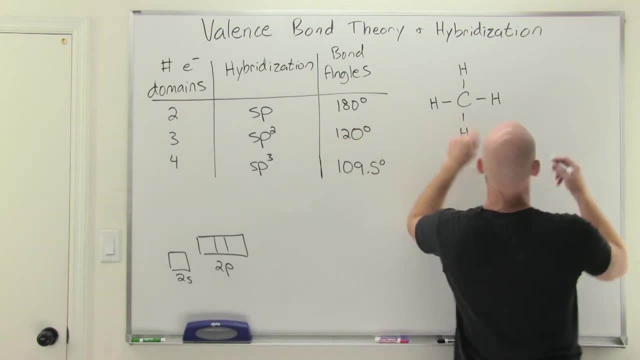 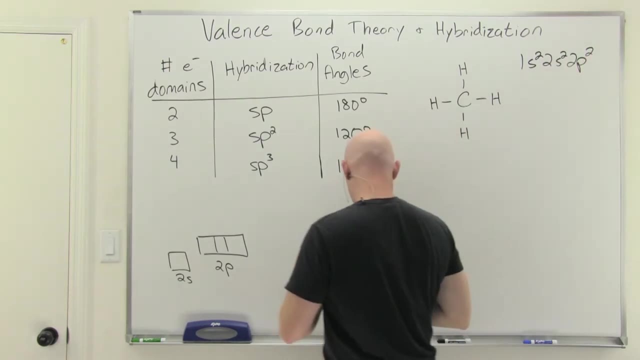 all explain that it's the valence electrons that are used in bonding. So if we take a look at carbons electron configuration, it's 1s2, 2s2, 2p2.. And if we kind of show that in diagram form, 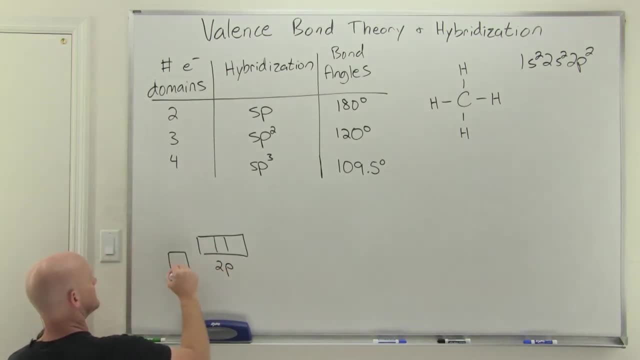 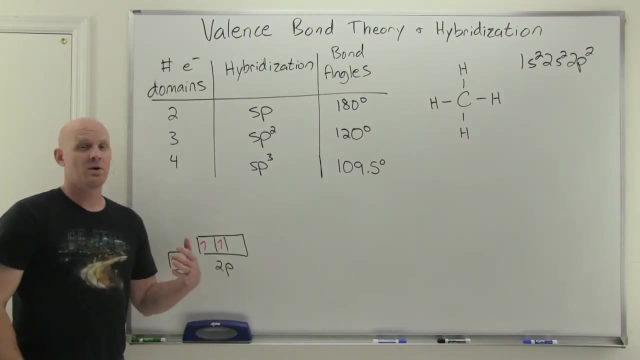 here we're going to focus on the 2s and 2p electrons, because those are the valence. So we've got two electrons in the 2s orbital and then we've got two unpaired electrons in two different 2p orbitals. Now classic bond theory say that it's the unpaired electrons that are going to bond. 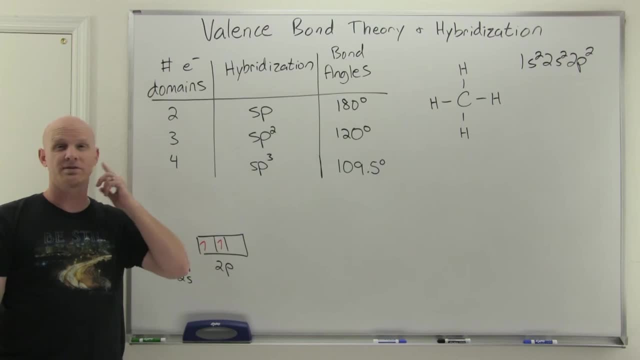 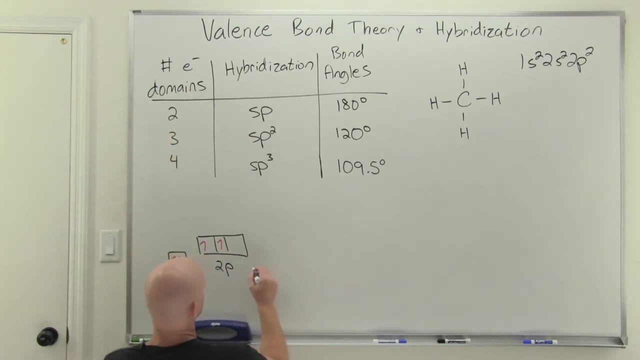 They're used in bonding. And so we look at this and say, well, carbons only got two unpaired electrons. Therefore, carbon should only be able to make two bonds. but we know that carbon makes four bonds, So there's problem number one. So there's an easy solution to this problem: Carbon is. 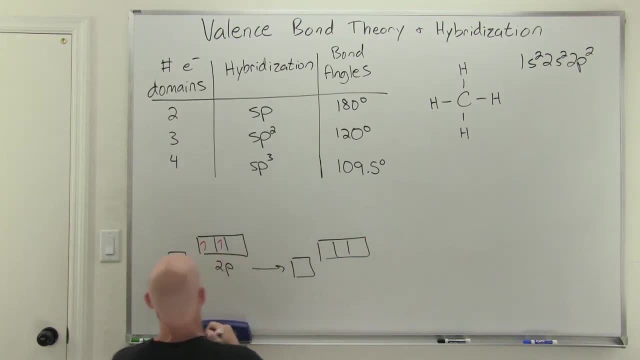 going to promote one of the 2s electrons and put it up into a p orbital And we call this a promotion. The result is that carbon now has four unpaired electrons and now can make four bonds. So when electrons are shared in a bond, that lowers their energy and makes them significantly more stable. 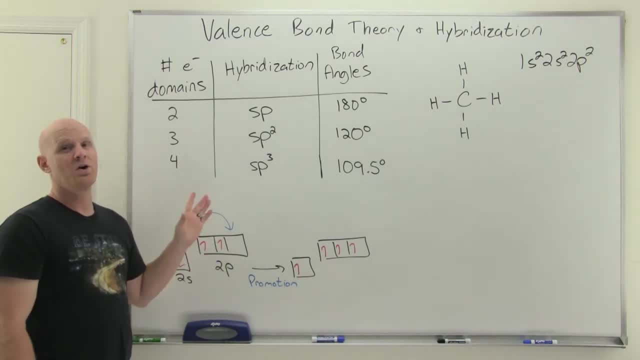 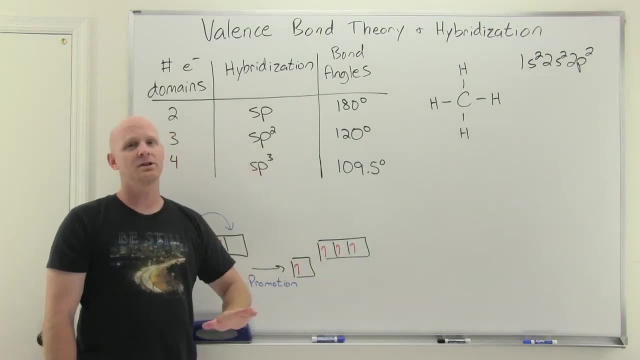 And so you might be like: well, Chad, why would this electron go to a higher energy orbital? Well, it looks like that's really just going to be an investment, because now, by making two additional bonds, there will be a significant lowering, significant reduction in the energy. 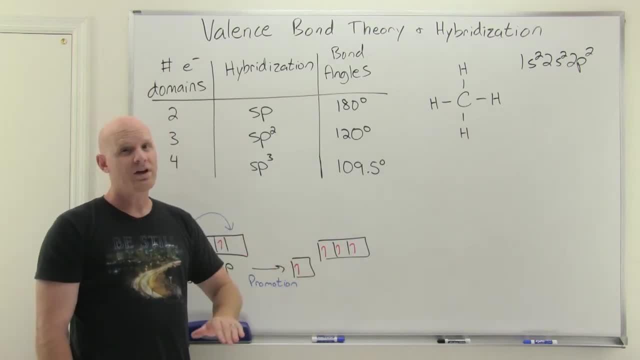 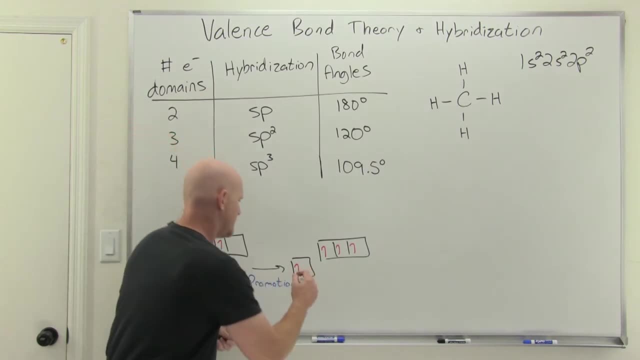 of the electrons So in the molecule and therefore it'll be a much more stable arrangement. So which is kind of the idea of why atoms make bonds to begin with. But we still have a problem here. So we've still got an electron in a 2s. 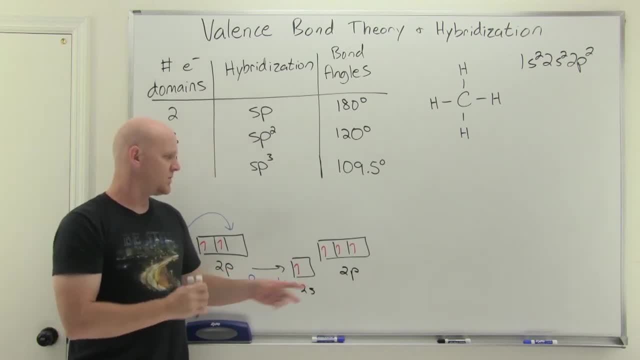 orbital and then three in the 2p orbitals. And, if you recall, those 2p orbitals are ones on the x axis, one's on the y axis, one's on the z axis And, if you recall, valence bond theory says that. 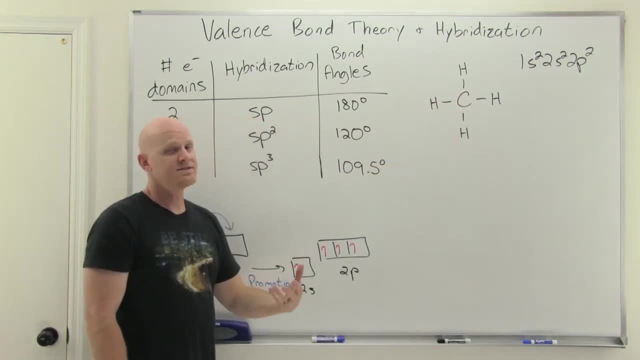 orbitals are overlapping to make these bonds. Well, hydrogen is a valence electron. It's only electrons in the 1s orbital. We know what he's going to be using to overlap in all four of these cases. The question is: what's carbon going to be using? Well, if we think this is what carbon's, 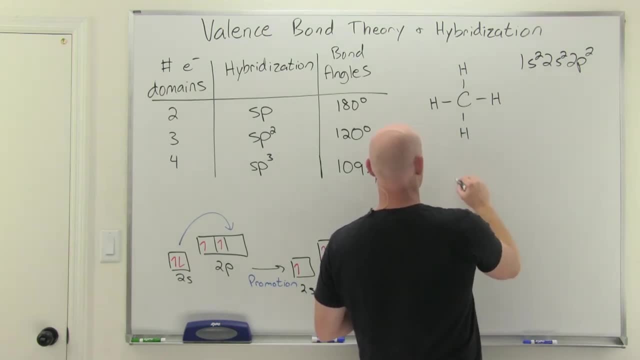 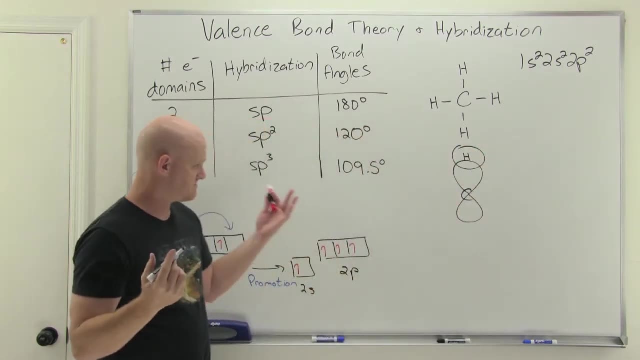 using, we're going to have an immediate problem. So let's say we've got carbon here with one of his p orbitals right there, And let's just say on top, that's where it overlaps with the s orbital of hydrogen. Cool. And let's say that's py Now. 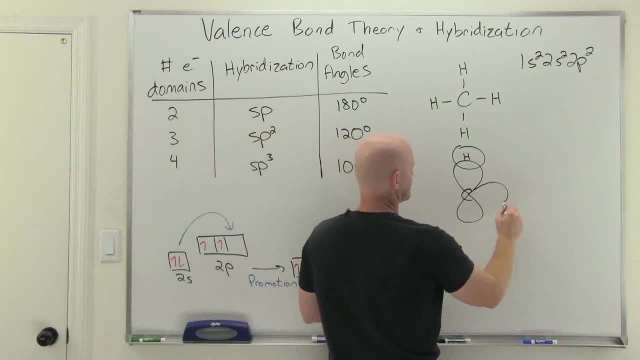 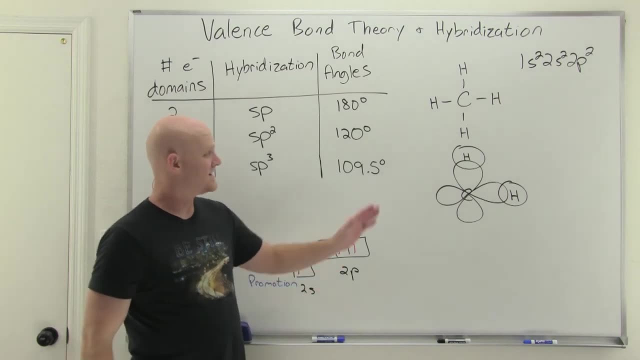 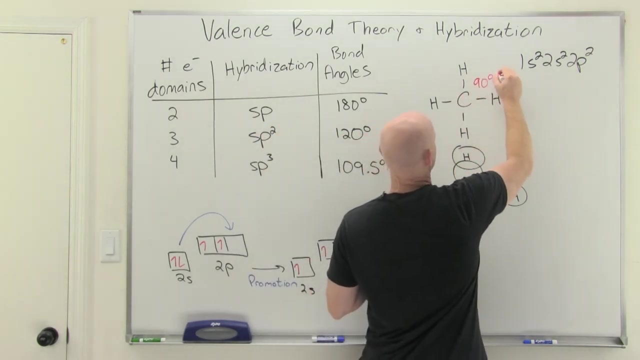 we take a look at, say, px, And px on the x axis overlaps with the s orbital of another hydrogen, And the problem is is that the y axis and the x axis are only 90 degrees apart, And that makes it appear as if the bond angles should end up being 90 degrees. 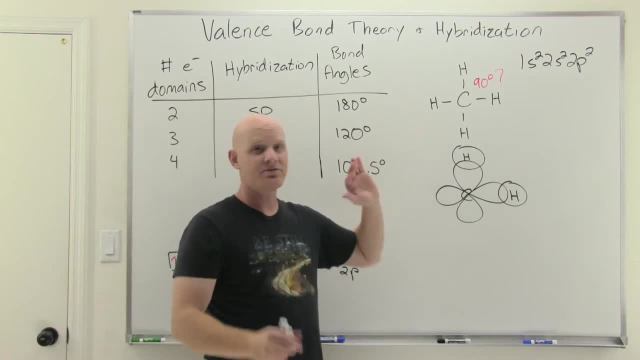 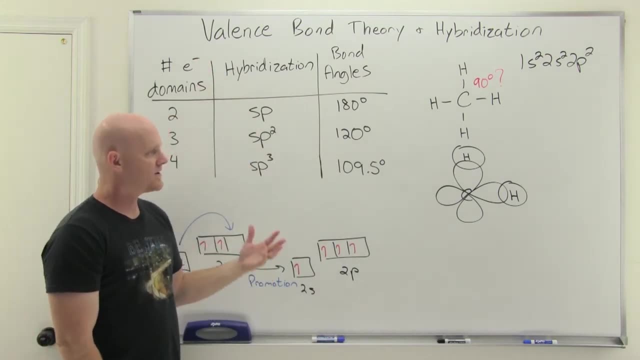 Except we know that they're not. We can look at a molecule of methane and actually measure the bond angles from electron density maps and stuff, And we know they're 109.5 degrees. And so what we figured out is that you know carbon's not actually using his s and p orbitals. 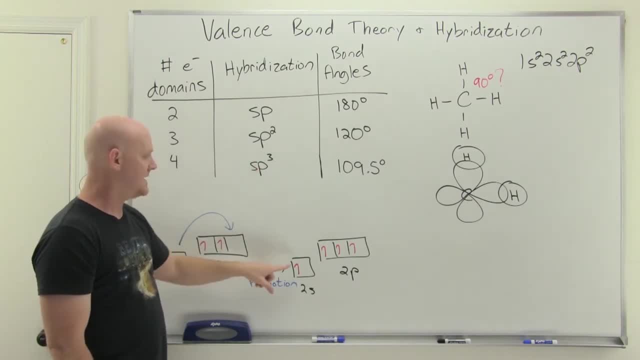 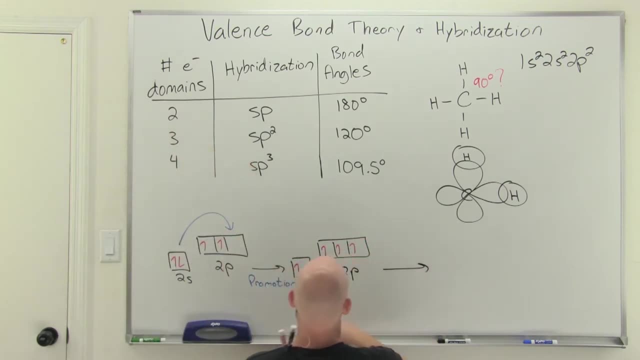 to make his bonds. What carbon is actually doing is combining these orbitals to make new ones, And so it turns out carbon is going to take and combine all of these four orbitals. So it turns out again: these orbitals are going to be 109.5 degrees apart, And so we know that they're not. 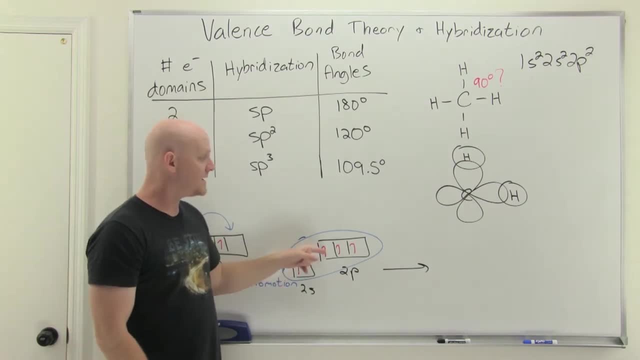 just math equations. They're wave functions And when you start combining math equations, well, you guys have combined math equations before, So we're doing something similar here. It's not quite so simple as that, but it's along those lines. But the number of wave functions you 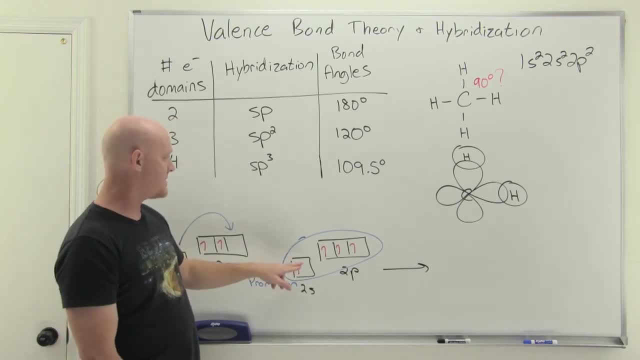 combine is the number of different ways they can be combined as well. So in this case I'm going to combine an s and all three of the p's. I'm combining four orbitals. It creates four brand new wave functions, four brand new orbitals, And since they're combinations of both s's and p's, 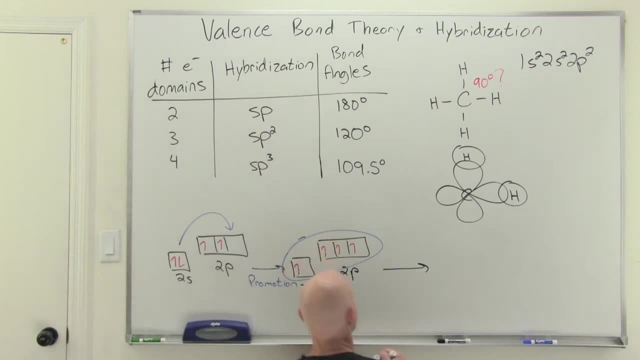 we'll call them hybrid atomic orbitals, And so in this case they're going to be a little lower in energy than p orbitals, but a little higher energy than the s orbital, since it's a combination of the two. We don't get crafty on the name, They're just based on what they're built from. Built from an. 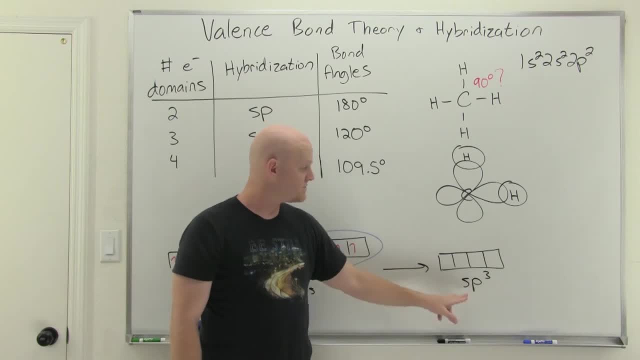 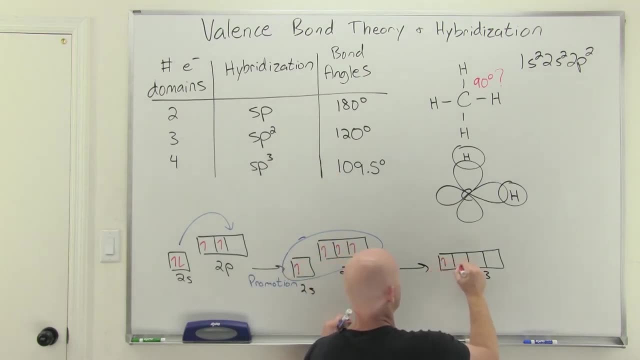 s and three p's, call them sp3s. So if you're sp3 hybrid types, you've mixed an s and three p orbitals, four orbitals total. You're always going to have four of these hybrid orbitals And these still all have an unpaired electron. So life is good. And now we just look at what. 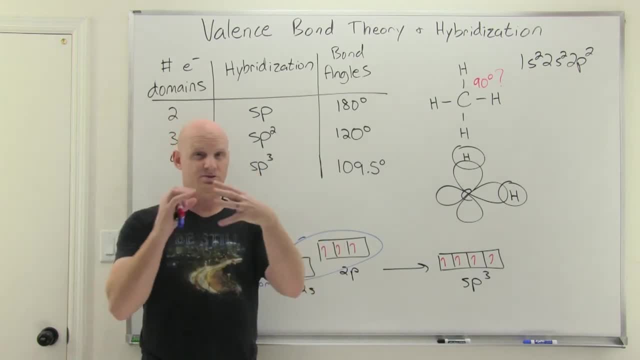 these are going to be, And we're going to have an unpaired electron. So life is good If we actually combine the mathematical wave functions, those equations, in four different ways. we call it linear combination of atomic orbitals, if you care. So if you actually map. 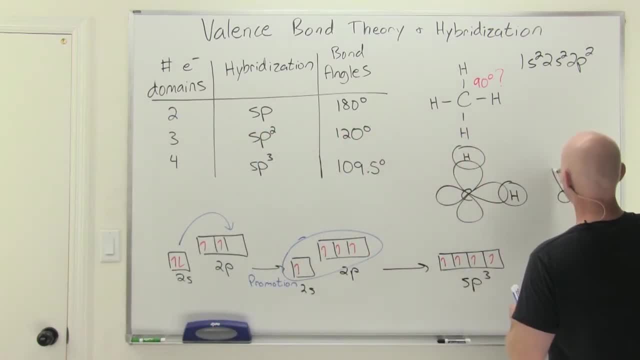 them out. so what you end up with is you got carbon and then you get this long kind of funky kind of orbital that looks kind of like a p orbital but kind of like with an extended s orbital, And it's a little bit strange but it's a combination of three p's and a single s orbital. 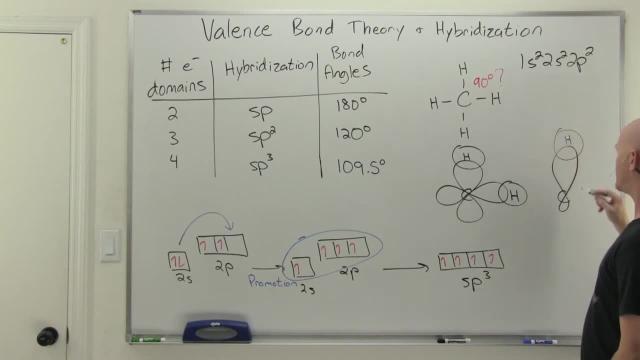 to make this And it can overlap with the s orbital of hydrogen. Then you get another one that would point down over here, And then you get another one that would point down over here, And then you get another one that would point down over here, down at an angle, And it turns out this angle, right? 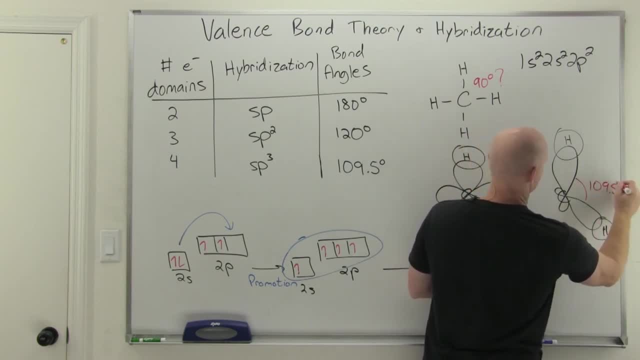 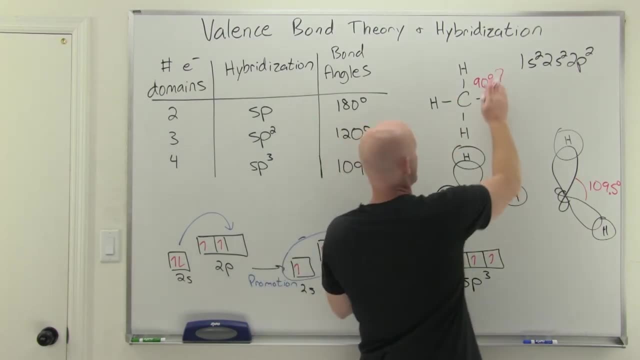 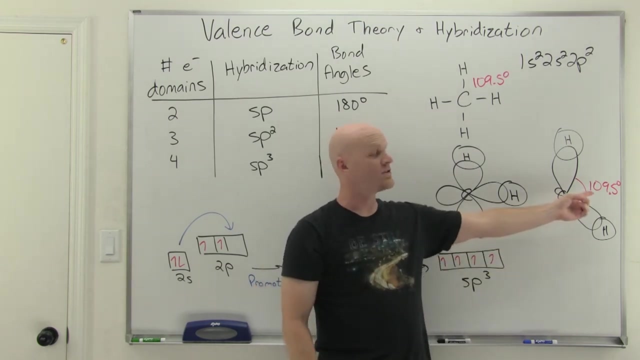 here is going to be 109.5 degrees Turns out exactly what we see in the molecule. It's not 90,, it really is 109.5 degrees, And the hybrid orbitals that we can create by linear combination of atomic orbitals are exactly 109.5 degrees apart. Now it's going to be difficult for me. 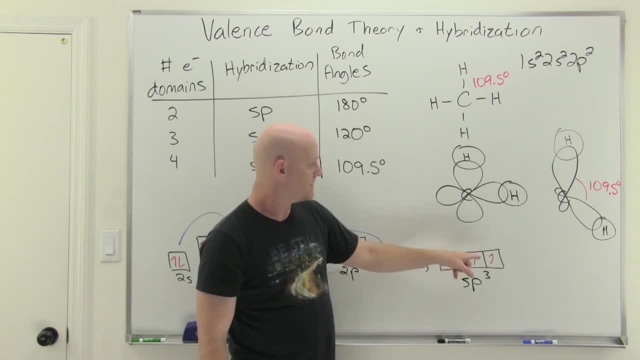 to draw the other two of these orbitals. I've drawn two of them. To draw the other two would be a challenge because they're not going to be the same. So I'm going to draw the other two of them, because it's a three-dimensional shape. One of them would be coming out of the board. 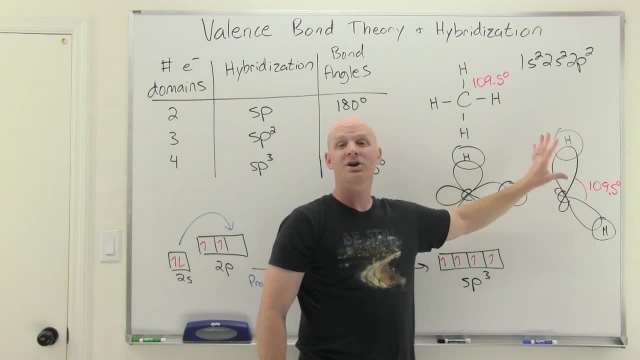 one of them would be going back into the board, But it would be a much better drawing if I could, but I've only drawn half the drawing here, So cool, But you get. the idea is that now this actually is a better reflection of what we see in reality for the actual molecule of methane than 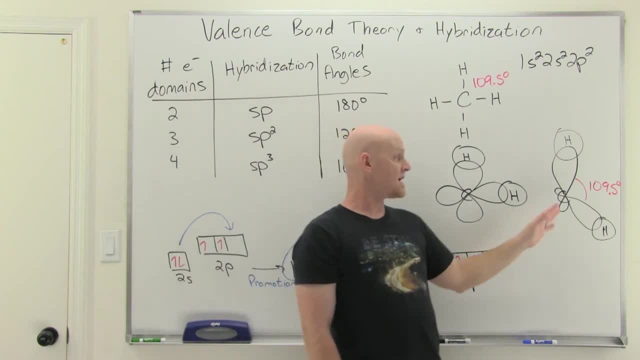 trying to use the original. just plain old s and p orbitals. Cool. Now it turns out that the truth is, though, this is kind of a lie as well. It actually is even more complicated than this. We talk about molecular orbital theory in the next chapter. 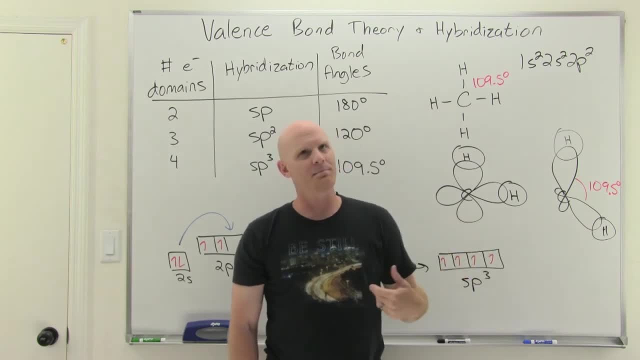 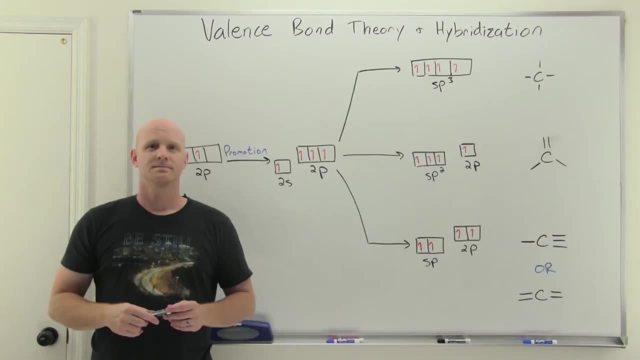 This idea of hybridization and stuff like that. it's not really a perfect reflection of the truth either, But we'll get closer to that in molecular orbital theory in the next lesson. So now we're going to take a little more thorough look at hybridization. We'll look at it from the 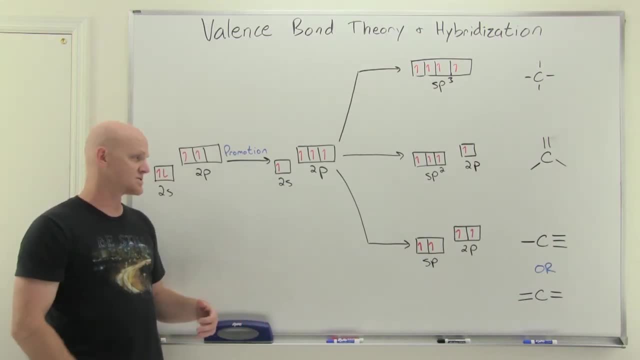 perspective of carbon being that this is organic chemistry. but this happens with other elements as well. And again, carbon has four valence electrons, only two that are unpaired. It promotes one, so that it now has four unpaired electrons. But we see, if we use these regular. 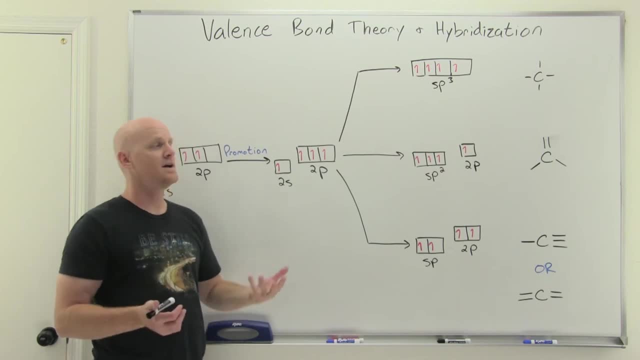 atomic orbitals, we don't get the right geometries that correspond to reality. And that's again the idea behind why hybridization, why that theory kind of took hold and why we suggest that it occurs. Now we got really three different options for carbon. in this case He can. 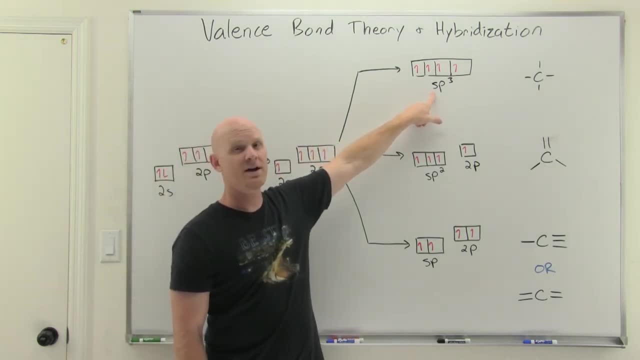 mix his s and all three p's and make four sp3 hybrids. That's one option, And if you have four electron domains, that's exactly what you want to do, because those sp3s all point 109.5 degrees apart. Now your other option is to only combine an s with two of the p's. And if you combine an s, 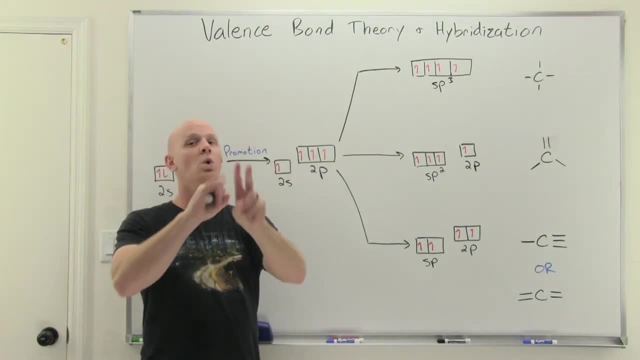 with two p's. one s, two p's, you're only combining three orbitals. You only have one s with two p's, And if you combine an s with two p's, you only have one s with two p's. And if you combine an s with two p's, you only have. 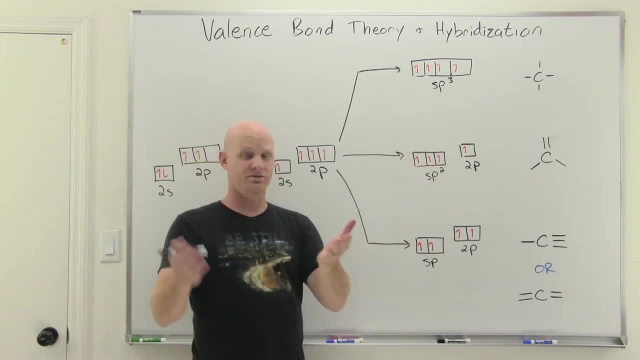 three hybrid orbitals And we call them sp2 hybrids just based on what they're composed of. But that leaves you with an unhybridized p orbital. that last p orbital- not part of the hybridization process at all- left behind still unhybridized. Cool, And that's perfectly the case. 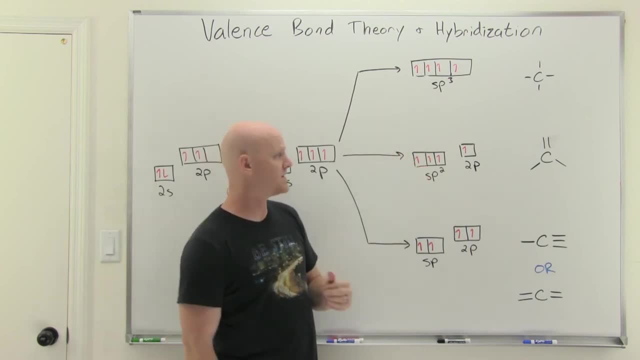 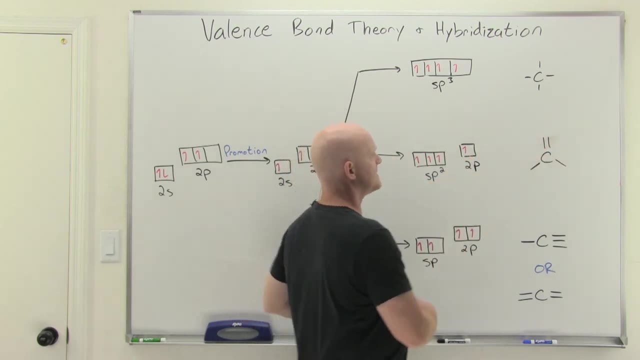 These sp2 hybrids, it turns out point magically 120 degrees apart, But the p orbitals left behind that electron right there, because that's what you'll need to make a pi bond. So keep in mind, in this kind of a structure where carbon's got one double bond and two single bonds, 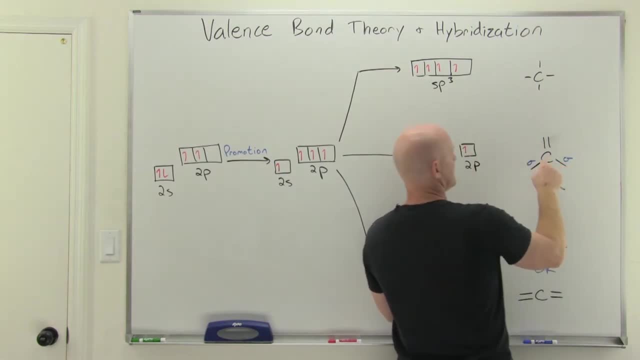 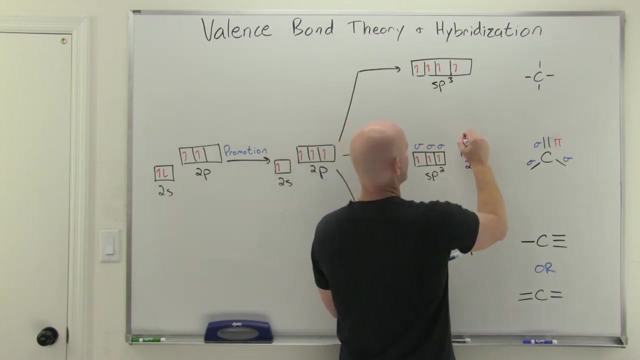 all single bonds are sigma bonds. So when you've got a double or triple bond, the first one is also a sigma, but any additional bonds past that point are going to be pi bonds, And so you can see that the hybrid orbitals are going to be used to make all the sigma bonds, but it is an unhybridized 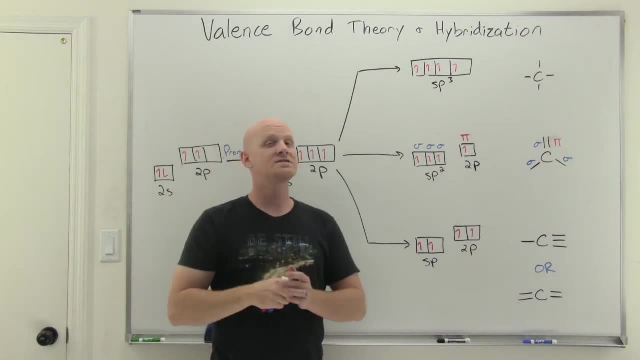 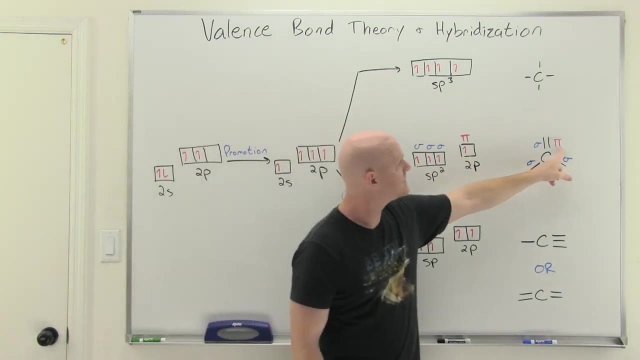 p orbital that is needed to make pi bonds. Keep in mind again that a pi bond is always the sideways overlap of plain old p orbitals. Nothing else can be involved in a pi bond. That's why we had to have a p orbital left over to make that pi bond. 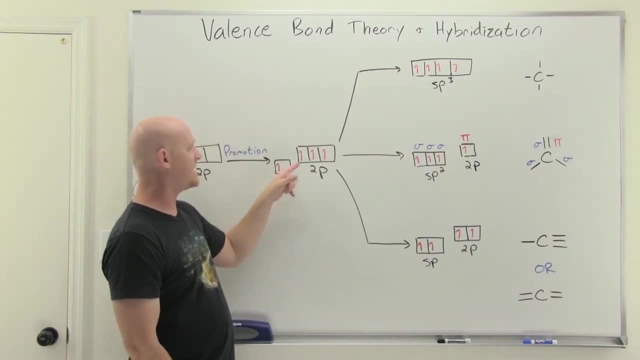 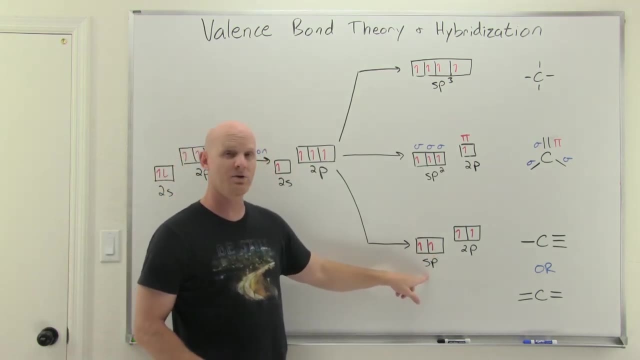 Cool. Now the last option is if we just mix one s and one p orbital. So if you mix a single s and a single p, you're only mixing two orbitals. You only create two hybrids. We call them sp hybrid orbitals. They magically point 180 degrees apart And that leaves you with the last two p orbitals. 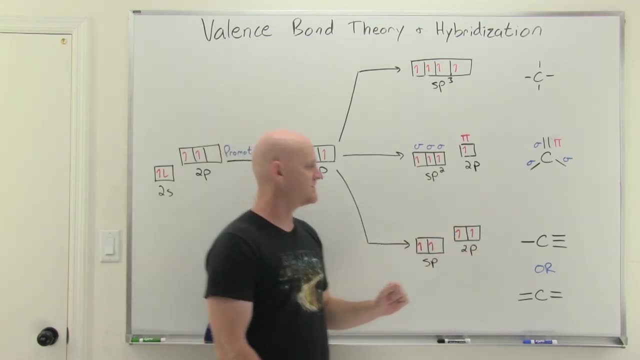 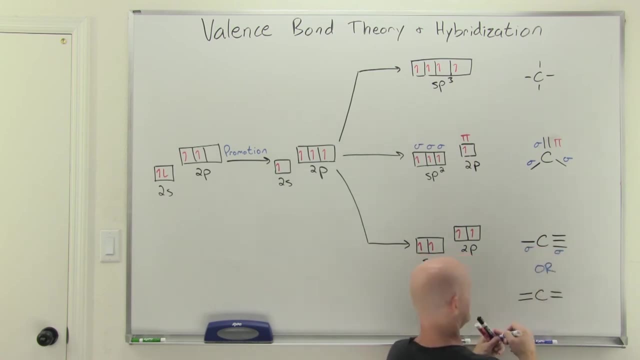 still in existence And they're used to make pi bonds. And so when you see a carbon having a single bond and a triple bond, again the single bond is a sigma bond And the first bond of the triple bond is a sigma bond as well, But the other single bond is a sigma bond. And so when you see a 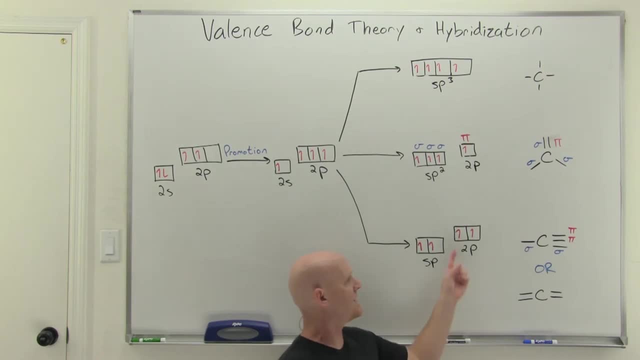 two bonds are both pi bonds And that's why we needed these two different p orbitals, one for making each of those pi bonds. This also happens. it turns out much less commonly but if carbon's got two double bonds. So the first bond on either double bond is a sigma bond, but the additional 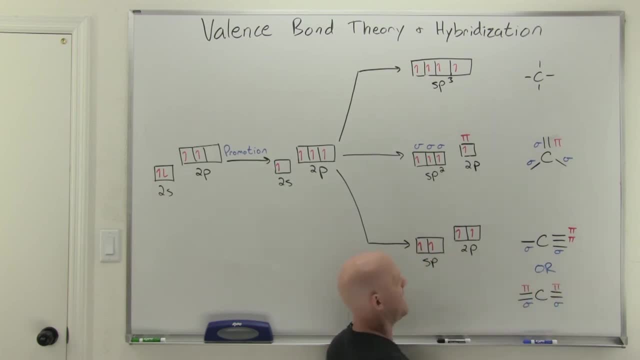 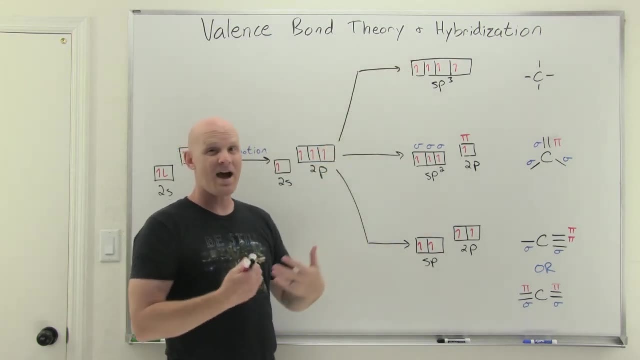 bonds are also pi bonds, But having a triple bond would be a much more common occurrence that you'll see throughout the course. Cool, But these are the kind of three results for carbon, And it just magically works out that with sp3, it's going to be a triple bond, And so we're going to have a. 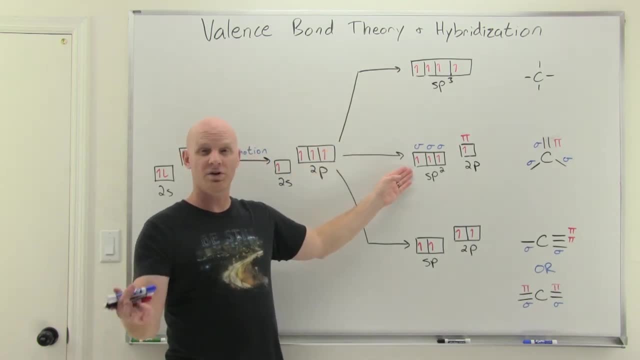 triple bond and it's going to be a super bond, And so with sp2 hybrid orbitals they're all 109.5 apart. That with sp2 hybrid orbitals they're always 120 apart, And with sp hybrid orbitals. 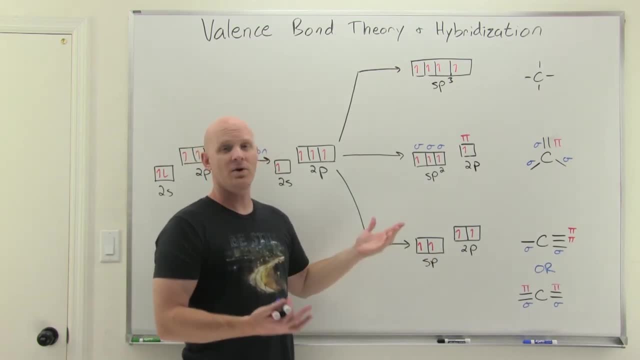 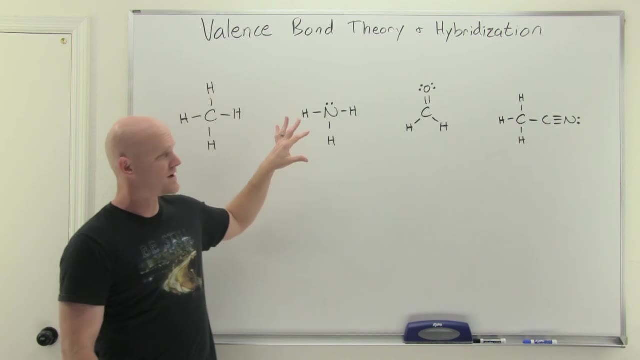 they're 180 degrees apart. So explaining you know how this matches up with what we know from VSEPR theory and how molecules really look Alright. so we want to visit these molecules we had on the board just a second ago And if you look at the study guide, they're in that as well. 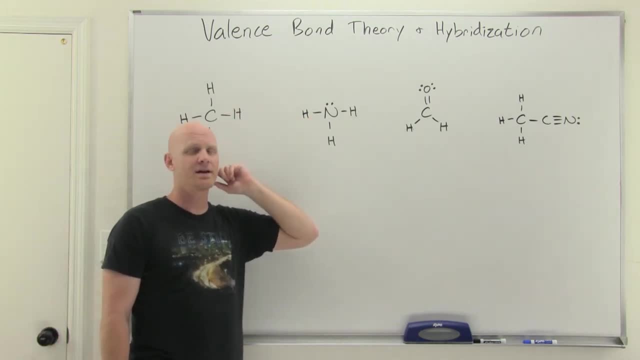 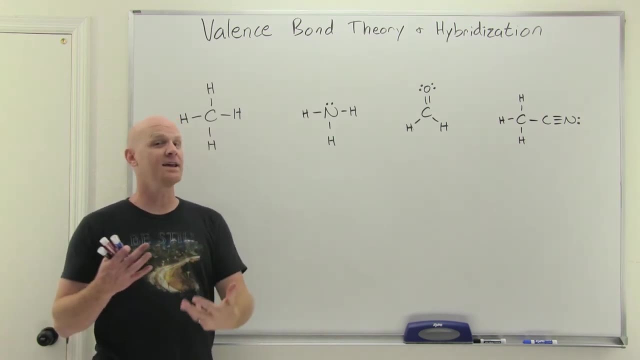 So we'll look at them one more time and talk about a common question you're going to see in an organic chemistry exam, And so what they might do, in light of everything we've just presented now, is talk about what orbitals are overlapping in any given bond or what orbital is a particular lone pair of. 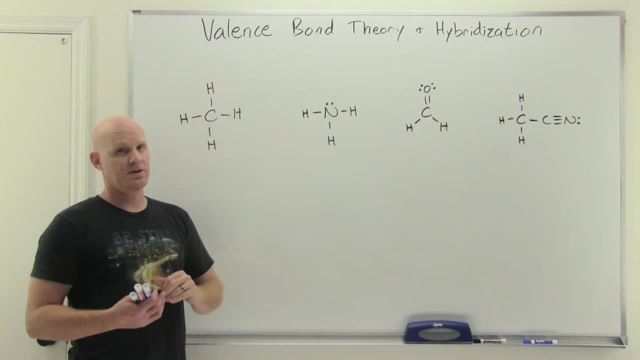 electrons in. So now, first thing I want to do is go back and, just you know, designate hybridizations for all these lovely atoms here, And so, in this case, carbon: right here is sp3 hybridized, having four electron domains. Nitrogen. here is also sp3 hybridized, having four electron domains Carbon. 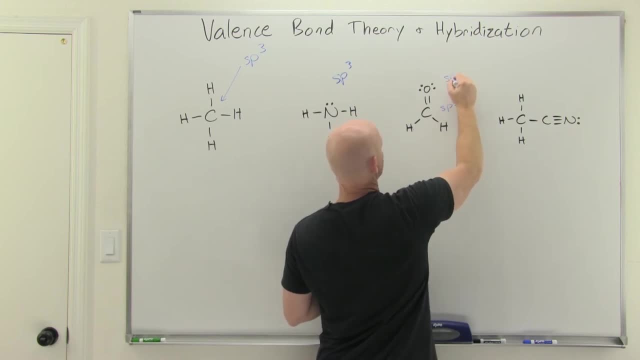 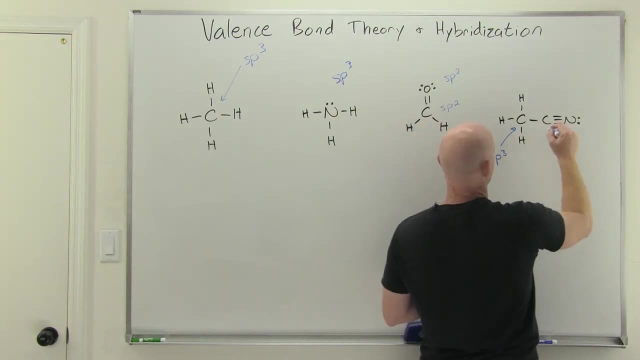 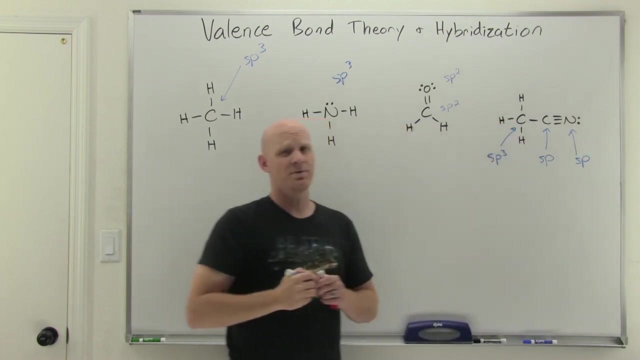 here is just sp2 hybridized. Oxygen was as well, both having only three electron domains. So the carbon on the left here is sp3 hybridized. So carbon on the right is sp hybridized, having just two domains. And then nitrogen, also sp hybridized, having just two domains. Now the way this works. 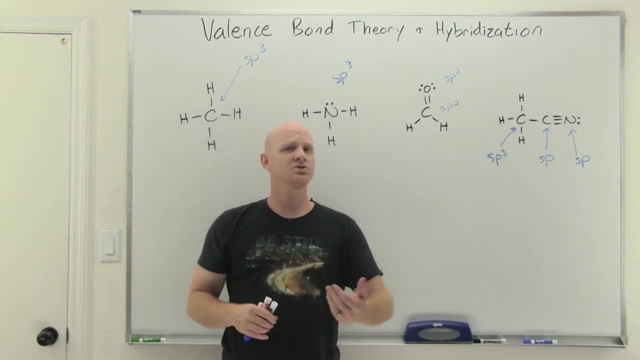 if an atom is hybridized, it will always use hybrid orbitals to make its sigma bonds. It will also put lone pairs in those hybrid orbitals as well. So if we take a look here, so carbon, here in this case, has four sigma bonds, one there, one there. 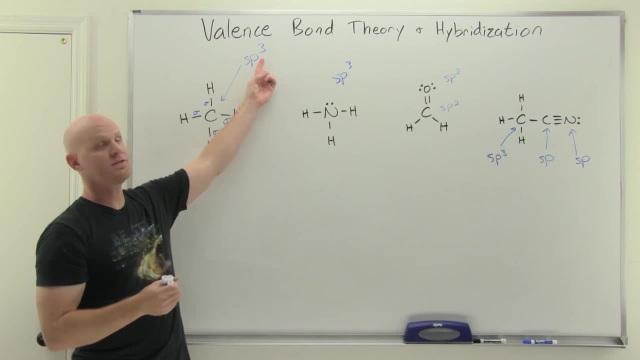 one there and one there, And he's going to use an sp3 hybrid orbital for his half of all four of those. Now hydrogen, on the other hand, is not hybridized at all. He's just got that one unpaired electron only going to make one bond, And when that's the case, he just uses the plain old regular. 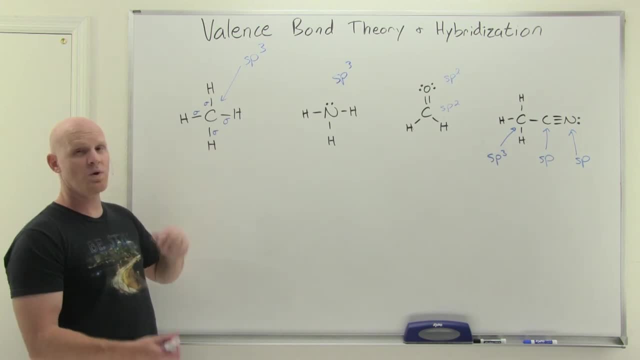 atomic orbital, not the hybrid atomic orbital. And for hydrogen that's just a 1s orbital. So if the question said, hey, for that bond right there, what orbitals are overlapping to create it, Well, carbon? you'd look at and say well, he's sp3 hybridized and that's a single bond. 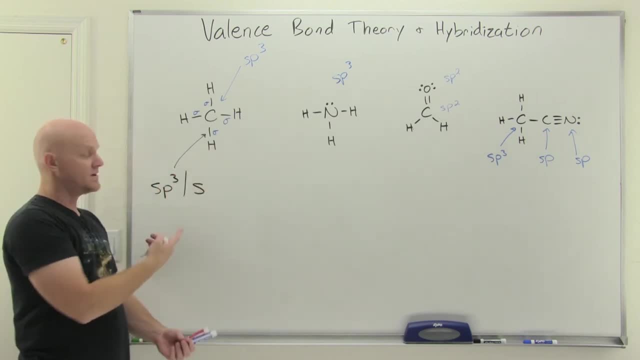 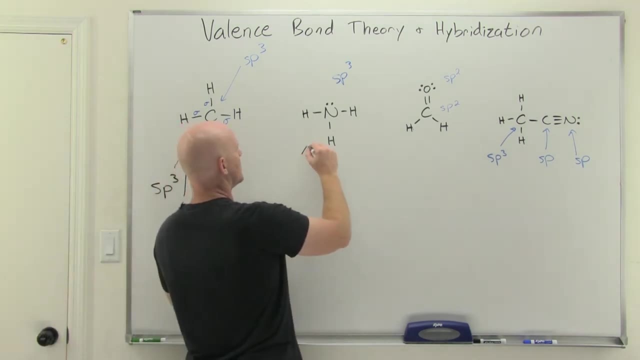 So he's going to use one of his sp3 hybrids And hydrogen is just going to use an s orbital, And those are the orbitals that are overlapping to create that sigma bond. Cool, If we take this a little further, we could also point at any one of these nitrogen-hydrogen bonds, and you should be. 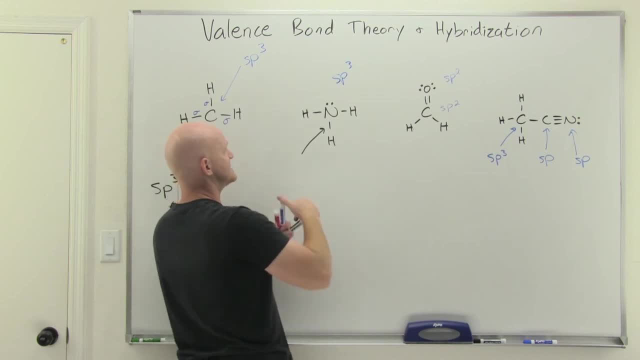 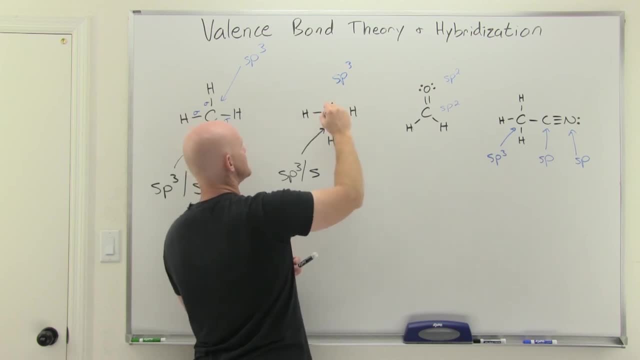 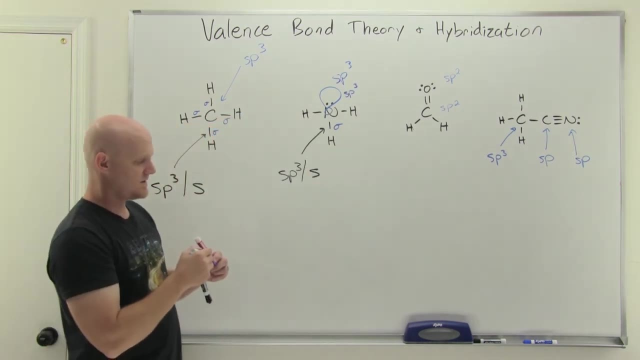 of hybrid orbital is this? Well, you could also be asked: well, what kind of hybrid orbital is that lone pair in? right, there And again, nitrogen is hybridized, And so he's going to put that lone pair in one of his sp3 hybrid orbitals as well. Okay, move on to the next one here. So if we were 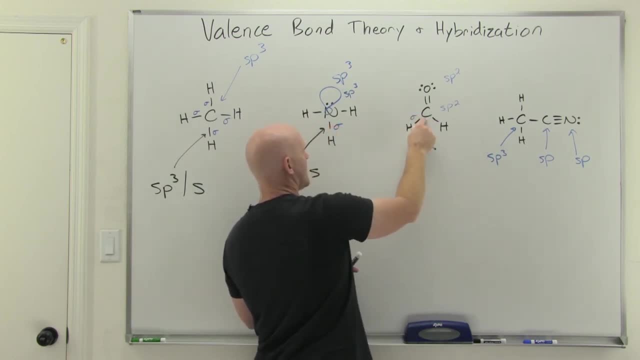 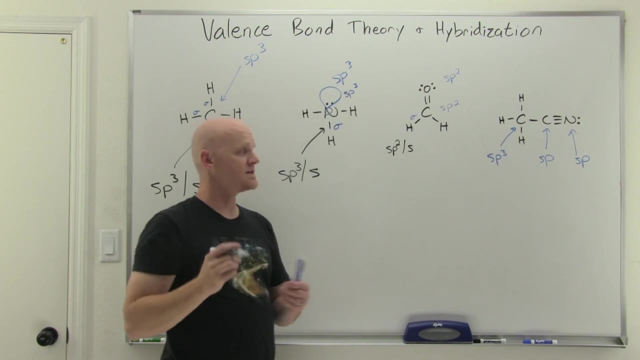 asked about one of these lovely sigma bonds between carbon and hydrogen, the carbon being hybridized. we'll use an sp2 hybrid orbital And the hydrogen just going to play and again use his s orbital. Now things get interesting if we look at the carbon oxygen bonds, because there's both a 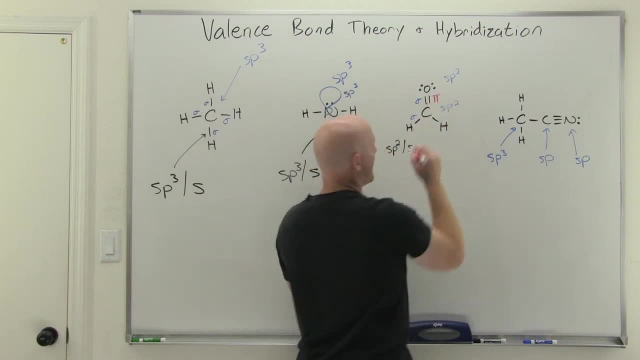 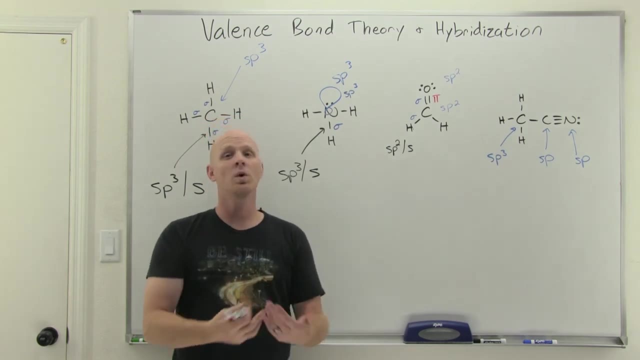 sigma bond as well as a pi bond And if you had your choice on which one you want to be asked about, you should choose the pi bond every time, Because if it's a sigma bond, any orbitals can be involved and you have to figure out which ones. But if they say what orbitals are overlapping to, 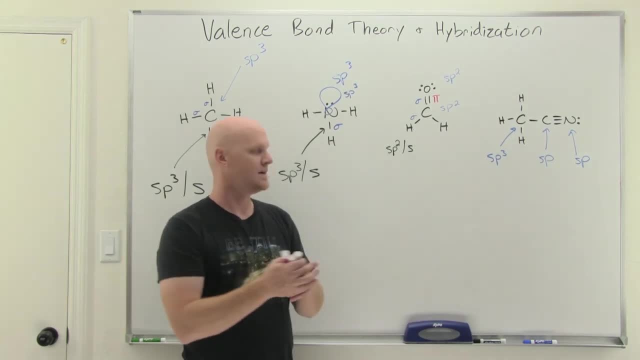 form the pi bond. you're just like P and P done Same two every time: P orbital with a P orbital, Carbon's got a P orbital, oxygen's got a P orbital and they're going to overlap side to side, not end. 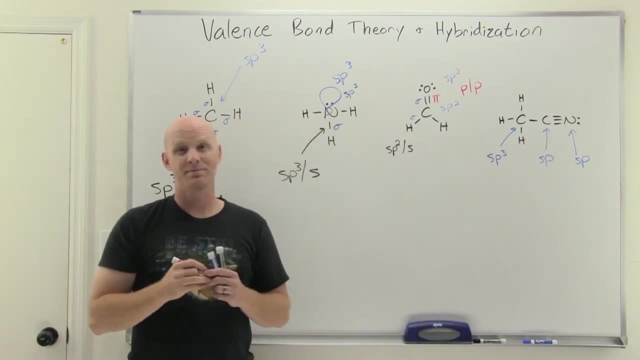 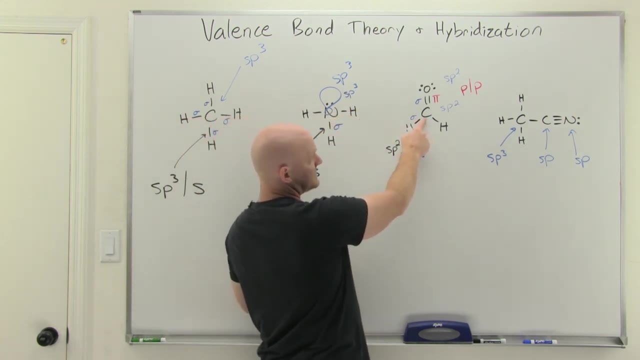 to end. But it's just going to be P orbital overlapping with a P orbital every time for a pi bond. So that's like the question. Now, if we look at the sigma bond, we'd have to say, okay, the carbon is definitely. 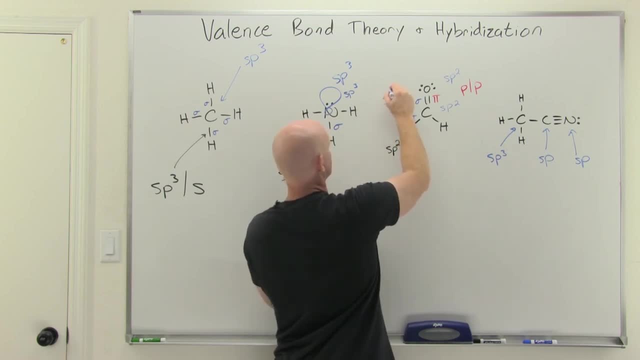 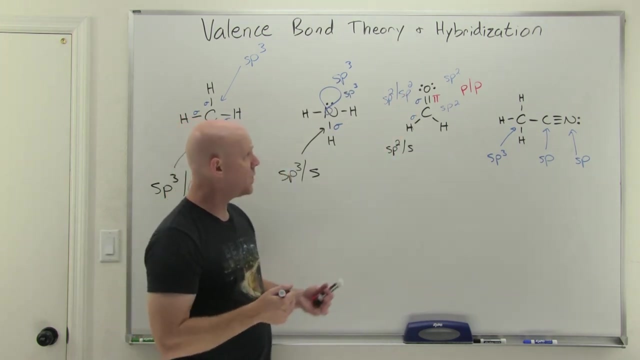 hybridized. So he's going to use one of his sp2 hybrids. The oxygen's also hybridized, And so he also will use a hybrid orbital, another sp2.. And so in this case, to make the sigma bond between carbon oxygen, it'd be an sp2 from carbon overlapping with an sp2 from oxygen. Cool. 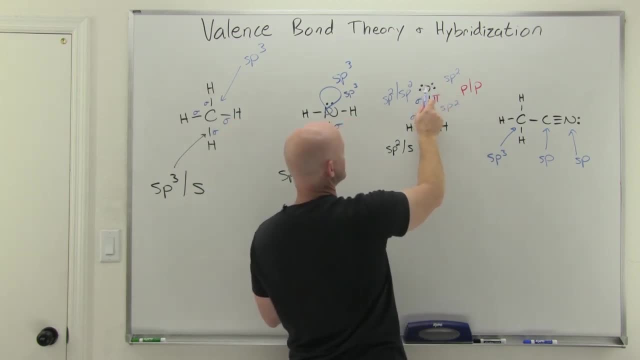 One more question we could ask is: what kind of orbital is either lone pair on oxygen in? And we have to say, oh, is oxygen hybridized? And yes, he is, He's sp2 hybridized. Then the lone pairs will both be in sp2 hybrid orbitals as well. Cool, And 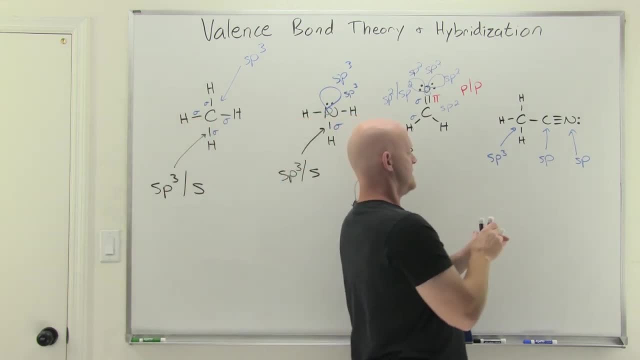 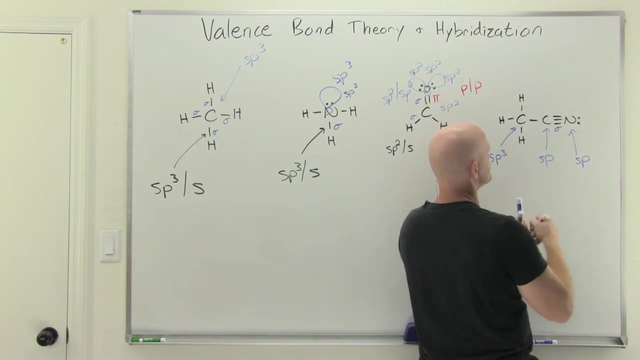 that's generally the way this works. Let's just look at one more example here. So if we look at that triple bond yet again, keep in mind that the first bond again is always a sigma. Any additional bonds past that are pi bonds. And again, if they said what orbitals are overlapping, to make either 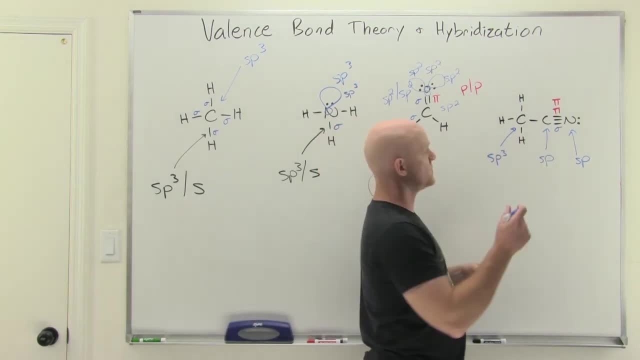 one of those pi bonds, P and P done. But my question for you is what orbitals are overlapping to make the sp2 hybridized? And if you look at that triple bond yet again, keep in mind that the sigma bond. So in this case we've got to look and say: well, carbon's sp2 hybridized The